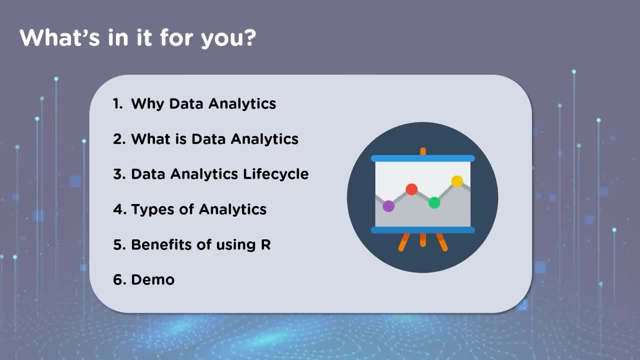 the basics. we will focus on why data analytics and the importance of data analytics, and then, what is data analytics? we will also focus on understanding the lifecycle of data analytics and I also try to give you some real-time examples so that we can relate these concepts with the 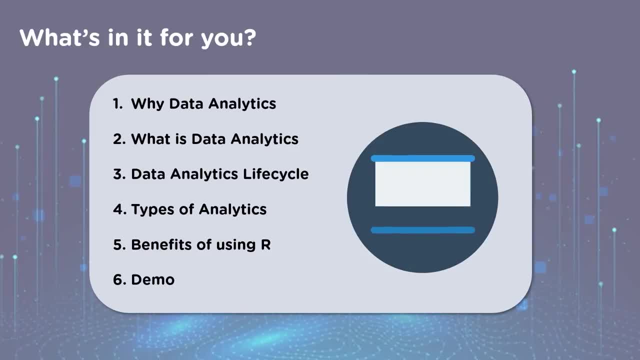 real-time examples or scenarios, and then we will understand the types of analytics and what do they mean. we will also focus on the benefits of using R. for this session, we will be using our studio tool. hence, we have to understand why we use R for data analysis and finally, we will perform. 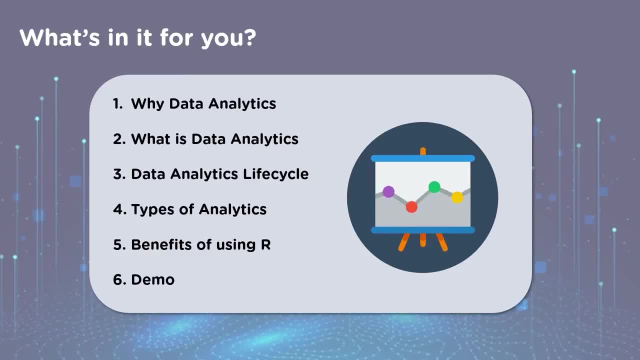 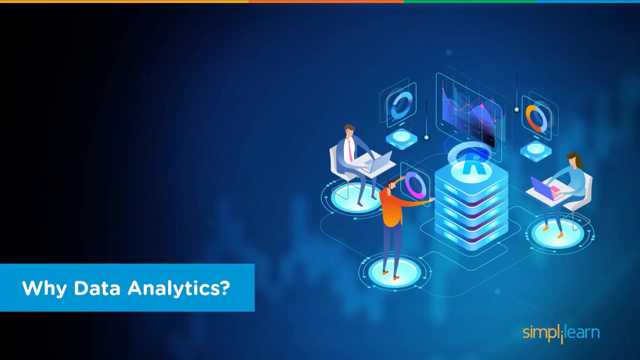 some hands-on exercise. in today's session, we will only focus on how to import the data, how to structure the data and also how to create some beautiful visualizations by using our studio. all right, so firstly, let us understand why data analytics. can somebody here tell me why data? 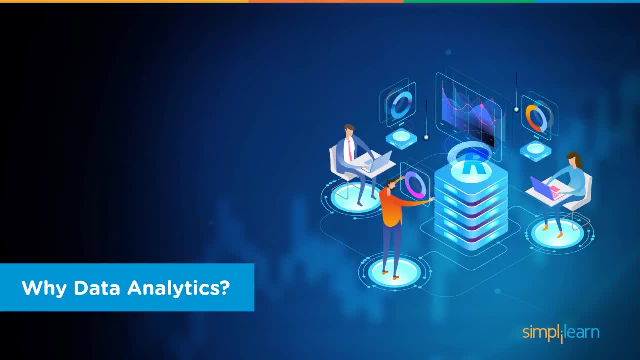 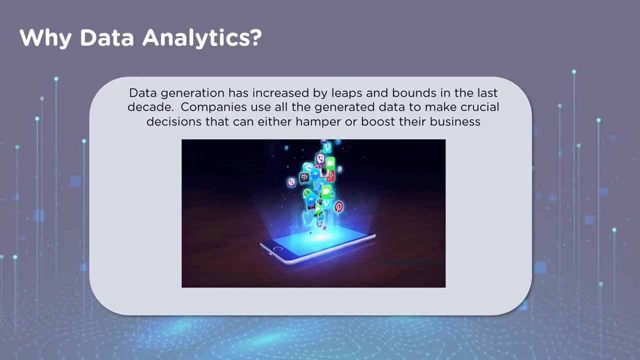 analytics and why is it used in organizations. so let us understand why data analytics and what is the use of data analytics. as we all know that data is growth going exponentially year over year, it is collected and it is also available everywhere. data is no more just available in structured format, but it is also available in semi-structured and 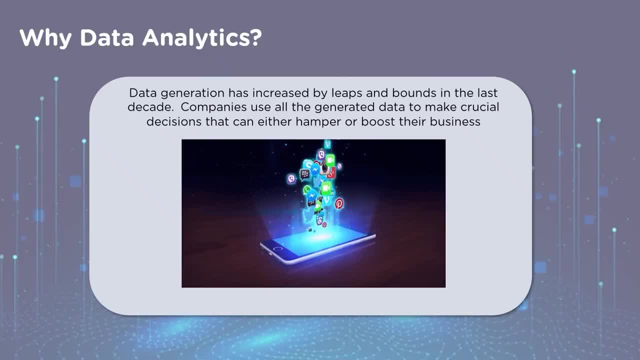 unstructured format. I'm sure you would have come across this term called as sentiment analysis pretty often, right? what does that mean? can we perform that in data analytics? yes, right, we use some natural language processing models, try to identify what are the good reviews, what are the bad reviews spoken by the customer correct? so we try to classify the text based on. 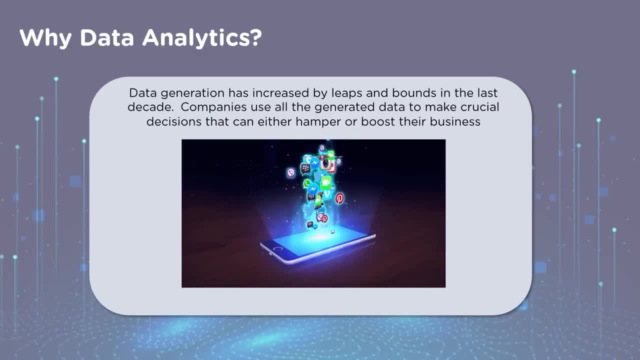 the good, bad and the neutral. so that is what sentiment analysis is about. so for that, to perform that activity, we have to also do some data analytics. now that companies have realized the importance of these information, not just structured but also unstructured data format, companies have started. 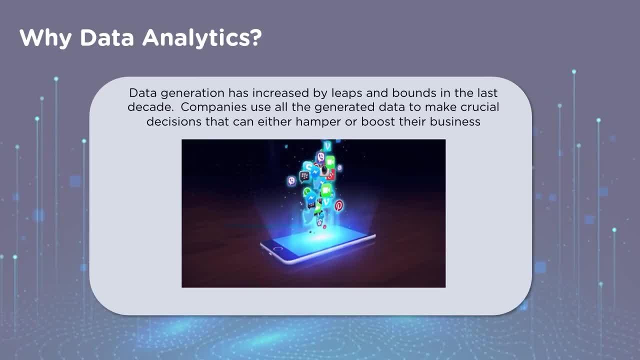 utilizing these data to take some crucial business decisions which can boost their business and also which can increase the efficiency of the business. so now that the raw data is accessible to the organizations, it becomes very important that the data is also stored well. I'm sure you all have pretty much heard about data warehouse in the last few decades. 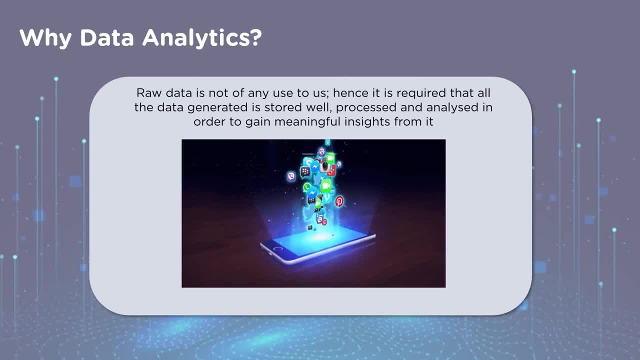 the trend was mostly on the data warehouses, the business intelligence tools. so the data warehouse used to collect these data, pre-process the data and also filter the data and make it available in a structured format for further analysis. however, now that is not the scenario. a firm coined as data Lake is available, and many firms are utilizing data Lake because it is a 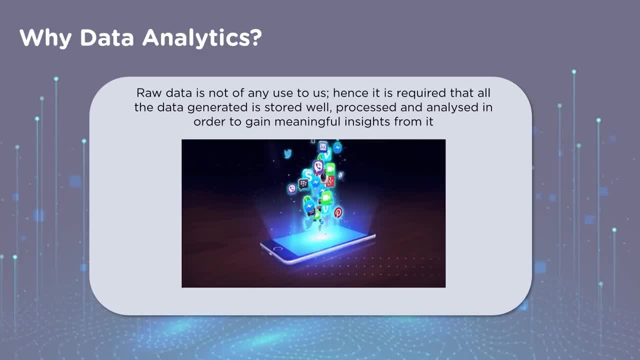 central repository which stores the raw data in form of structured and unstructured data. and now let us take a scenario. let us choose one of the participants here, Mark. so Mark has recently joined an organization as a data editor, as a data analyst or, in essence, a data scientist. the business connects with him and says that Mark. 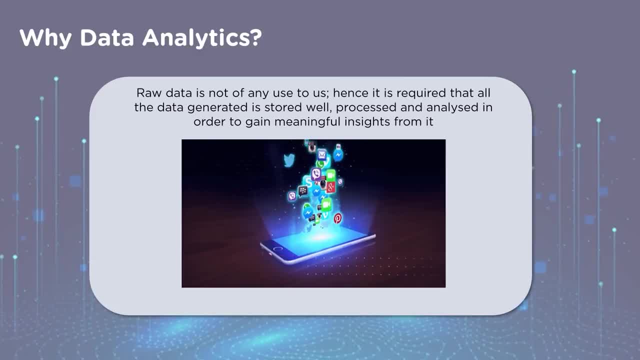 we have a business problem for you and we expect you to provide us a data analytic solution. so Mark sits with the stakeholders and he listens very carefully to the business question. so the business question says that we have couple of products which are performing really well in the market and 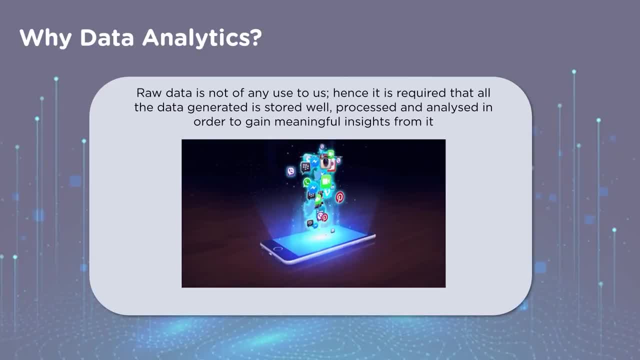 we see higher sales, some of the products are just not catching up in the market and we experience lower sales. can you help us identify what are the factors driving this higher sales and the lower sales? now Mark has to think with the data scientist mindset and be prepared to ask them right questions. 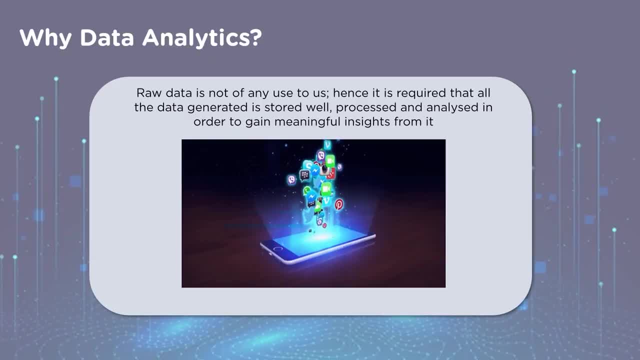 some questions such as: do you have the price of all these products available in the data data database And can I also know what is the duration of data availability? And also, Mark can ask some questions such as: do you also have some features of these individual products already captured in? 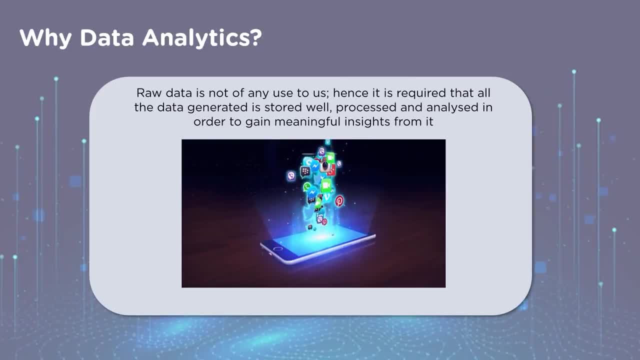 your database. So these are some of the interesting questions. that makes sense to the business, and the conversation continues, Which also means that data is not only information. Data analysis is about unlocking insightful information from this raw data, And hence data analysis plays an important 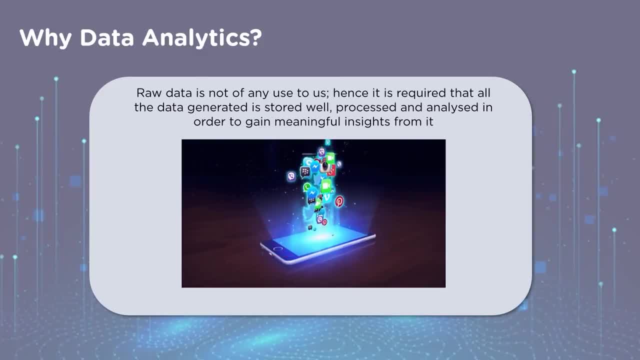 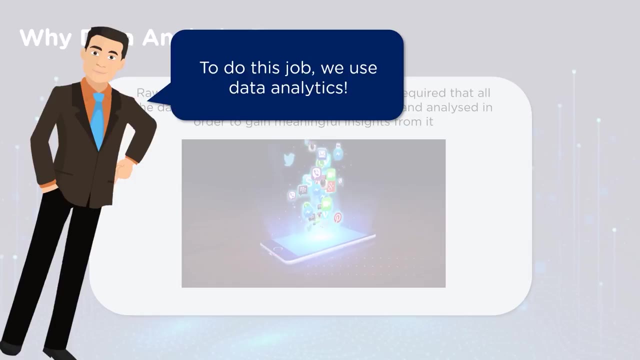 role in discovering insightful information, asking questions or answering the right questions, and also predicting the future or the unknowns, And to perform all these activities we use data analytics. So are you all with me? so far, Are we on the same page? Yes, Great. Now the question is: 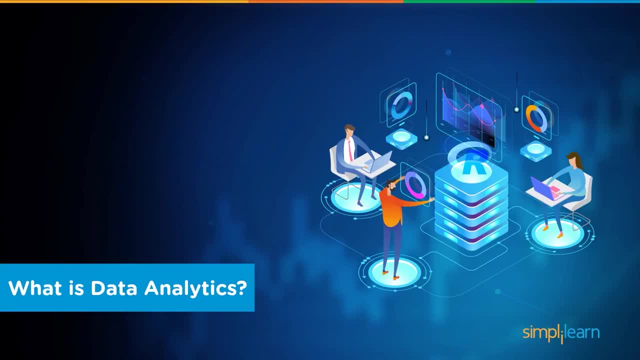 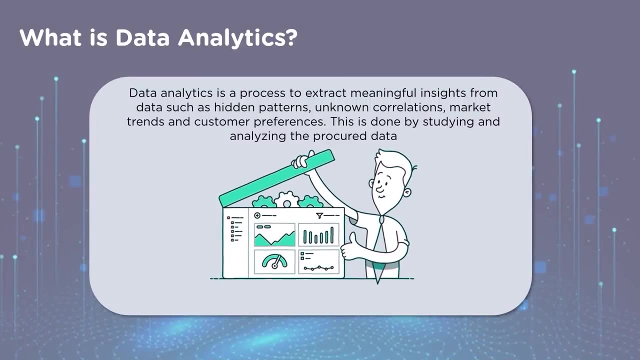 what is data analytics? So can somebody tell me what is data analytics? So let us see what is data analytics. We understood why data analytics and the importance of it. But perform any activities, there has to be a process, right. So data analytics is a process to extract. 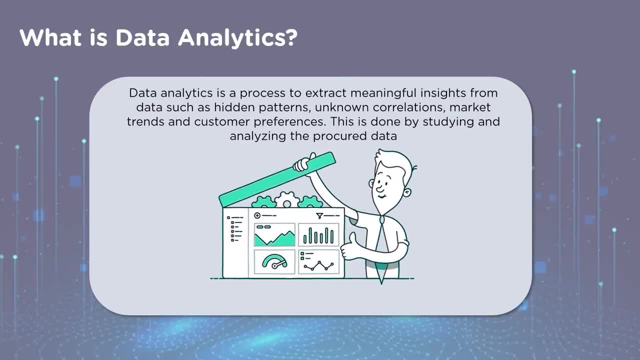 meaningful insights from data. Now let us continue with the scenario of Mark. So Mark now understands the business problem And he has also started asking questions about the data analytics. And here he is asking some relevant questions to the stakeholders, And he has also got the answers. 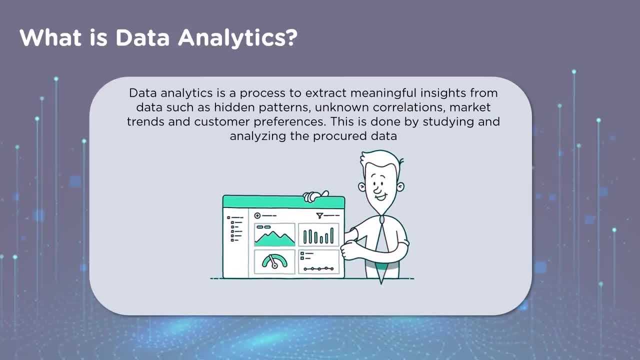 in return, He may start thinking about what could be the suitable solution for this. He may have to perform some exploratory data analysis to unlock some hidden patterns, to identify some correlation between the variables and to also know which are the key variables in the data set, And he may also 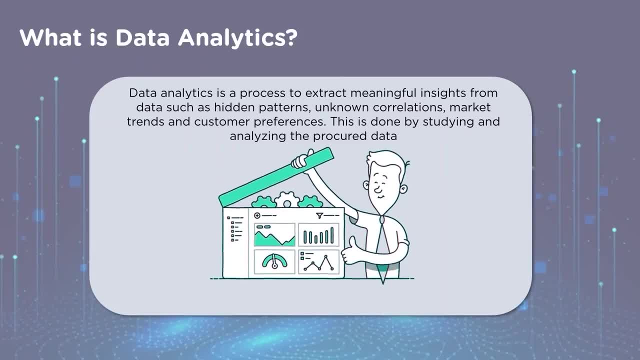 have to view the market trend, which means he may have to see that how the sales has been performing across the years or across the months. there might be some insightful information there. he may see that the sales has been growing exponentially for some of the products and some may be volatile. some may have some seasonality. 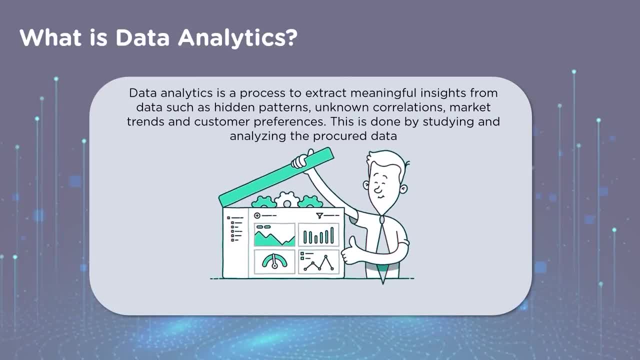 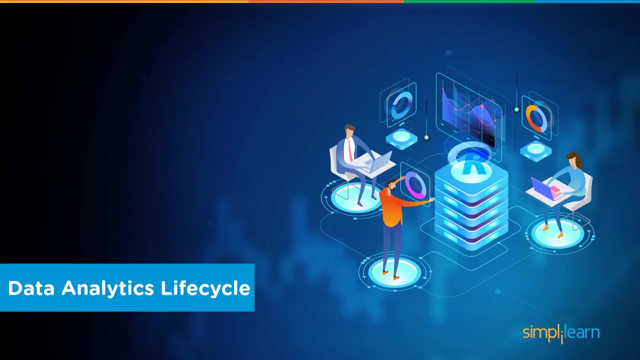 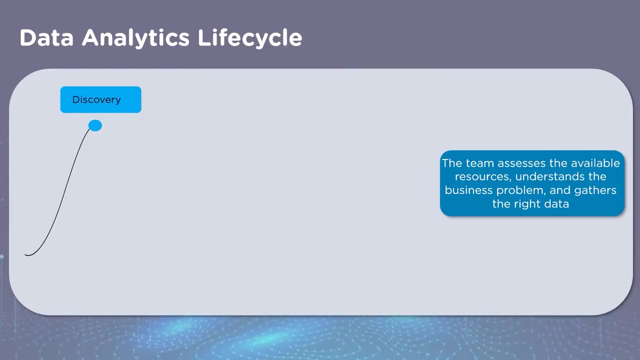 pattern or a cyclical pattern, etc. and also he may have to focus on the customer preferences- why are the customer reviews? and do some sentiment analysis. so now let us understand what are those life cycles of data analytics. we will begin with the discovery phase. this is the first phase. now that mark. 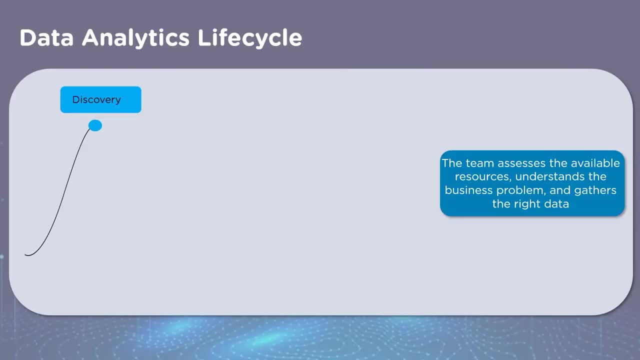 has understood the business problem, he will also start focusing on identifying the resources, that is, the customer preferences and the customer reviews. the data resources: some may be internal data resources that is available within the firm could be some transactional data, and some external data sources may be via web scrapping, identifying and capturing some competitor price on the. 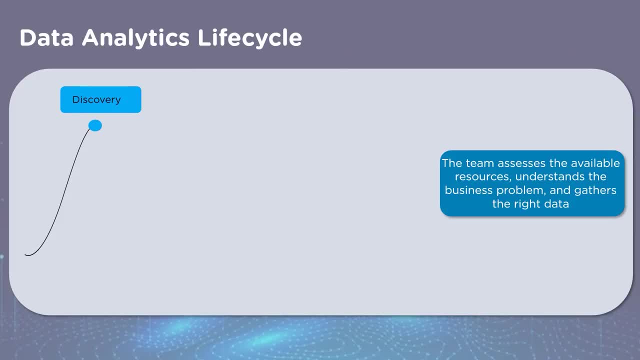 products. after gathering all of these right data, mark will focus on data preparation, which is the next phase. now mark, either individually or along with the team, will start focusing on the data preparation, which includes data wrangling, which means cleansing the data, imputing the records if there are any missing values or, you know, he may also. 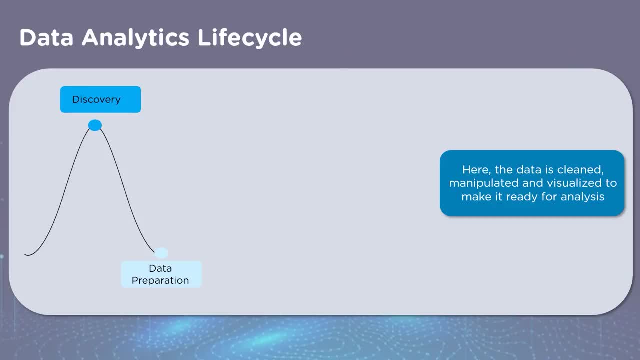 go ahead by removing those records if they are not required, and also doing some exploratory data analysis, which can include some statistical analysis, like looking at the data distributions, understanding the summary of this data distribution at individual variable level, doing some bivariate analysis and also trying to, you know, figure out which are the important variables that might. 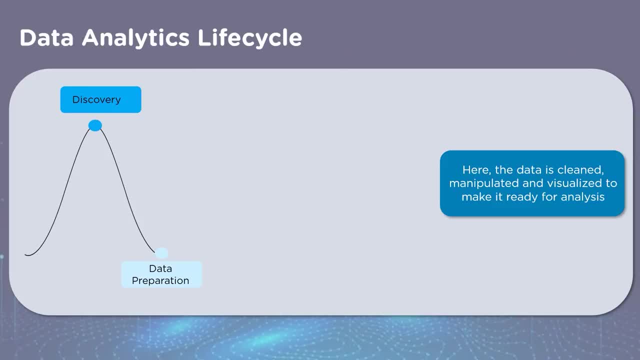 be required for the model building phase. after performing all of these EDA activities, which also include some visualization, mark will now sit with his team and try to identify the suitable models. the suitable models could be simple statistical techniques, or it can also be some machine learning models. so let's say that mark and his team has identified some five models. 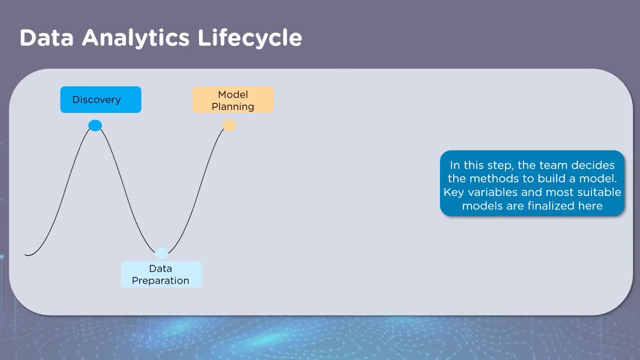 that can provide the required result, and out of these five models, they will filter down and they will prioritize the results that are required for the model building phase. now there are only three models that mark and his team have finalized. after this, they start focusing on model building activity. now for model building activity. 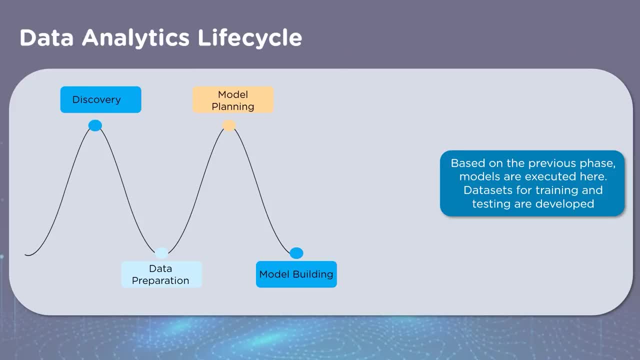 they have a data set already in place. so this data set will be split into training data set and test data set. it's not only training and test. we can also do some validation in between training and test. but here let's focus on training and test data set. he will 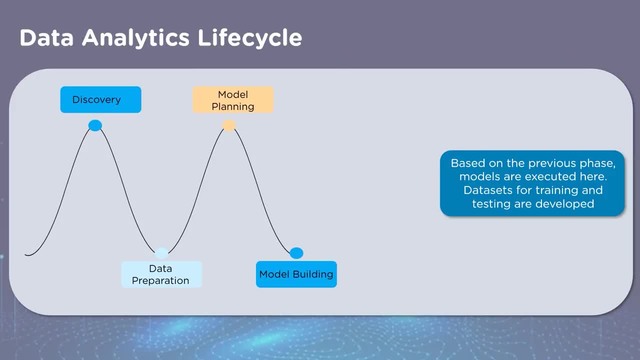 separate 75% of the data as training and 25% of the data as test. now, if your question is that, why perform this activity of splitting the training data set and test, can't we just go with one single data set? what happens if you just utilize one single data set? let us say that you have. 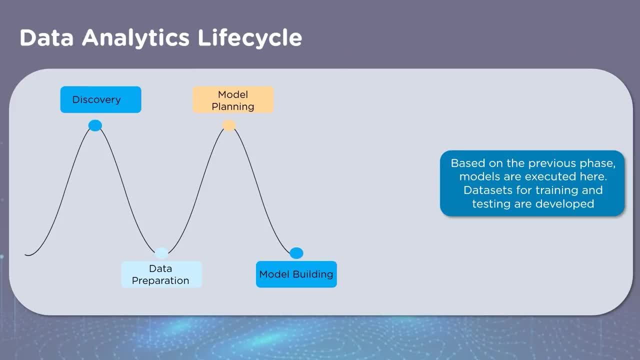 used the original data set and also executed this data in one of the selected model, and you will also observe the accuracy. let's say, the accuracy return is about 98%. 98% is a very good accuracy percentage and you may also be overconfident because of this. that may be a case due to overfitting. now what? 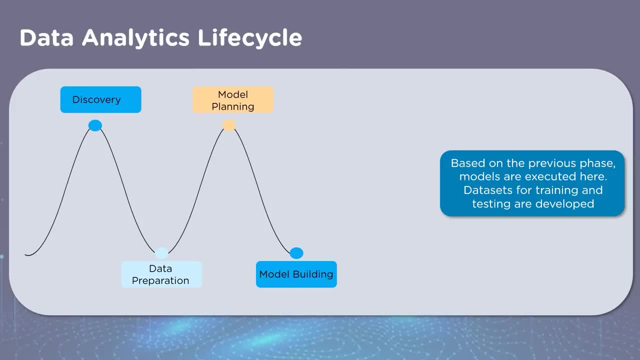 will happen when you add some new records into this data set and you rerun it. the executed model may not return you the same accuracy what you had seen. the accuracy might be 72%. now that's not fair. right to avoid these overfitting issues. 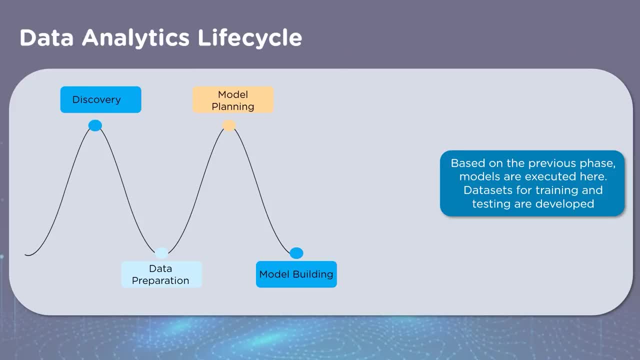 we ensure that some new records are tested separately. so hence we locate 25% of the data to the test data set and then we predict those records, the unknown records, which is located in the test data set. we predict them and then we test the accuracy of training data set and the test data set and we make a 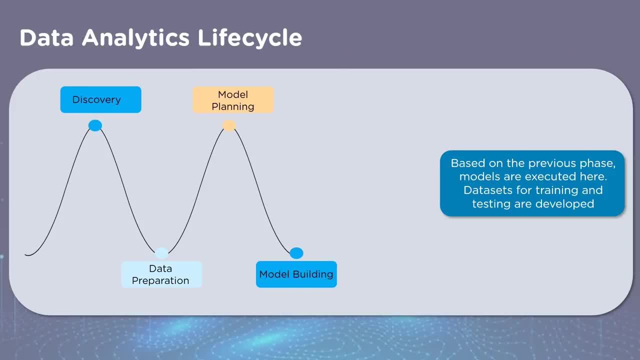 comparison. now let us say the accuracy result of training is 98% and the test is 97%. in this case we can say that the model is performing really well. however, while executing the model, there are certain things that has to be considered. for example, inclusion of the parameters tuning in the parameter which? 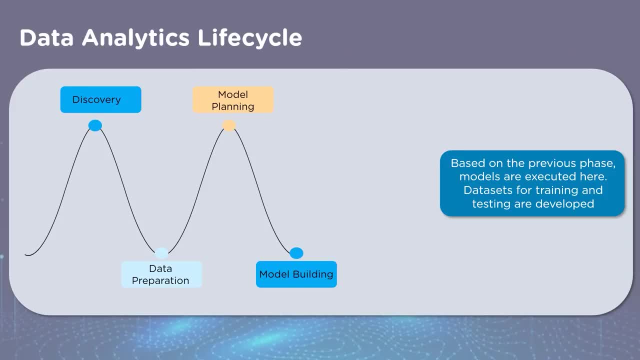 also will execute the optimal results. so this is very important to know that youたら. so this is very important. now, let's say, after performing this model building, the time comes to analyze the results. that is the next phase. now the team will sit and analyze the 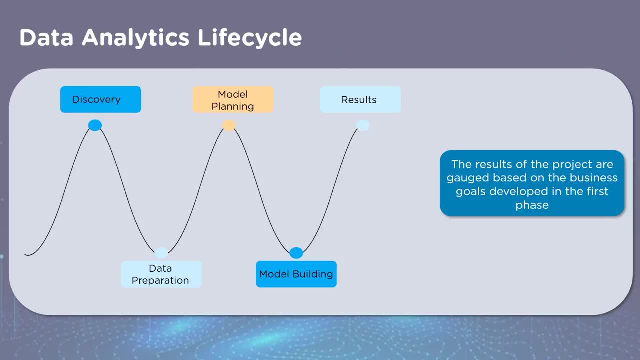 result and they will notice that out of the three filtered models, only two models are returning excellent accuracies. they will sit with the business team and they will also explain them the result and what are the activities that they have performed to obtain this result. some of the 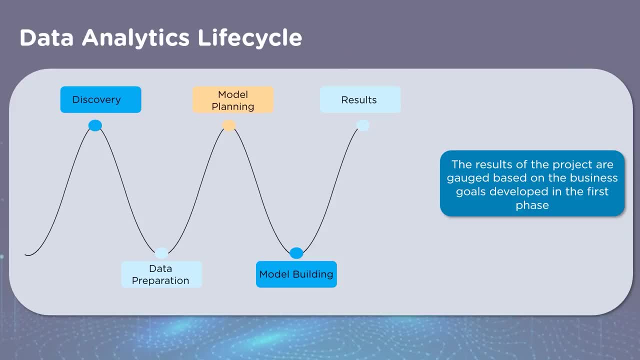 stakeholders may be technically savvy, some of them may be non-technical people, so it has to be very important that you also communicate these results accordingly. all right, now that you have the results, you will also gauge them based on the performance of the team, based on the results. 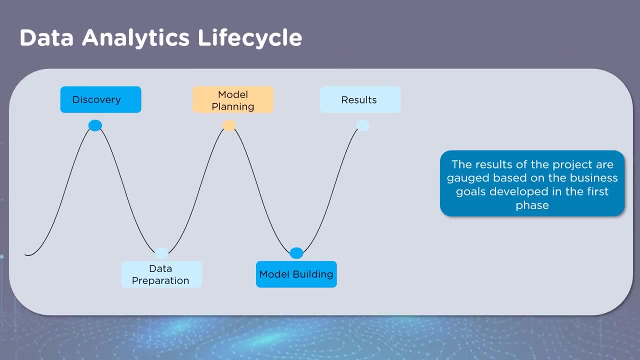 on the business objective which was developed in phase one. looking at the results of the two models now, the business might select one of the model and say that, okay, this particular model seems to be returning some right information and it also appears valid to us. let's go ahead with this one model. so 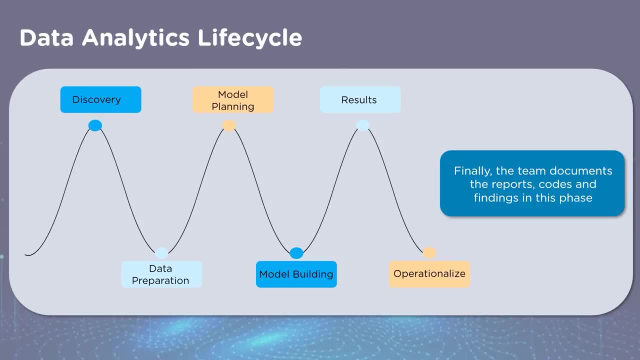 finally, the result and the model needs to be operationalized, and that is where the team will start documenting the business problems, the steps that were taken for executing the models, and they will include all the codes and the findings and, finally, they will implement this model so that the business can view. 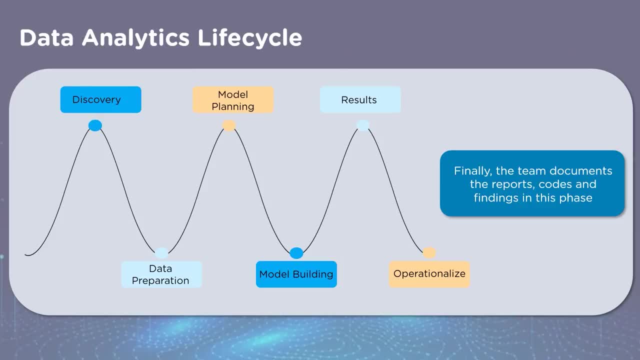 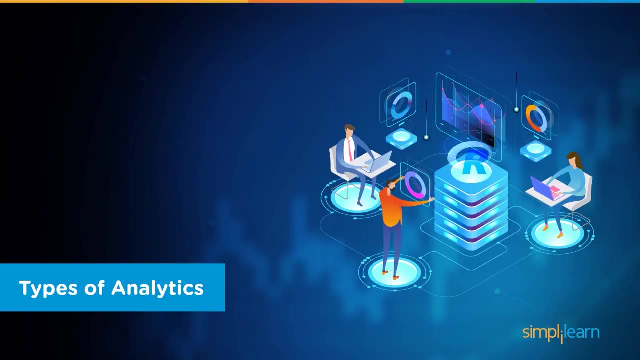 the results and also utilize them for strategic decision making at your firm. you so are we. good so far with the understanding of the lifecycle. all right, great. now let us focus on the types of analytics. what are the types of analytics? can somebody tell me which are the types of analytics you are aware of? 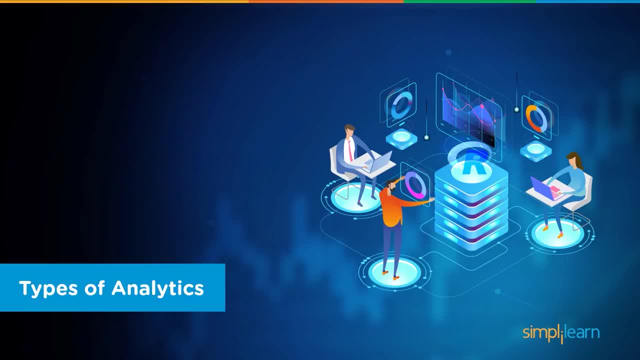 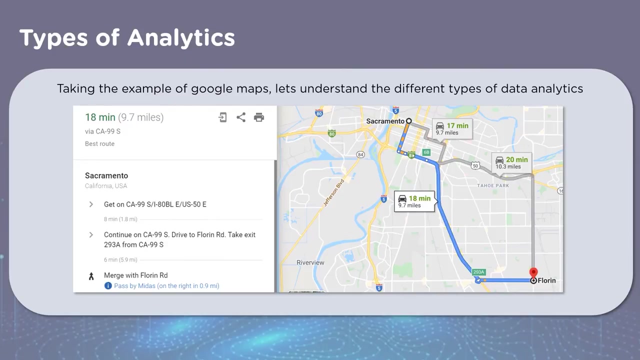 okay. predictive analytics- great descriptive analytics- good, all right. predictive analytics- great descriptive analytics- good, all right, good enough. now let us focus on this example of Google Maps. so as we look at this particular Google map, we understand that the blue color route is nothing but the route direction from Sacramento to Florin, and also we see a display of the 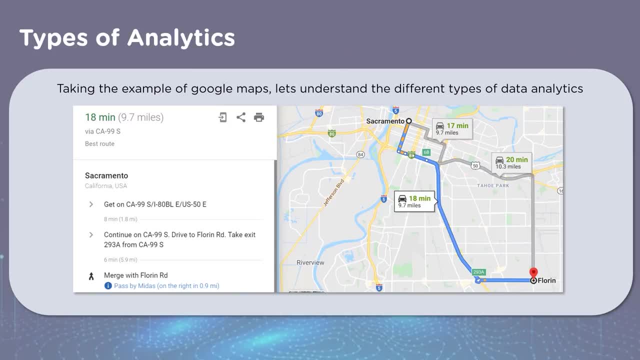 duration estimated as well the distance to travel from Sacramento to Florin as well. we see another route here that is gray colored. this is a substitute route or the connecting route, just to avoid the traffic which is in orange within the blue color route. so the gray colored route as well shows us the estimated. 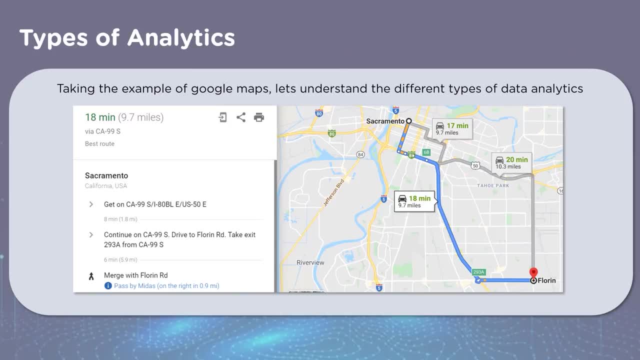 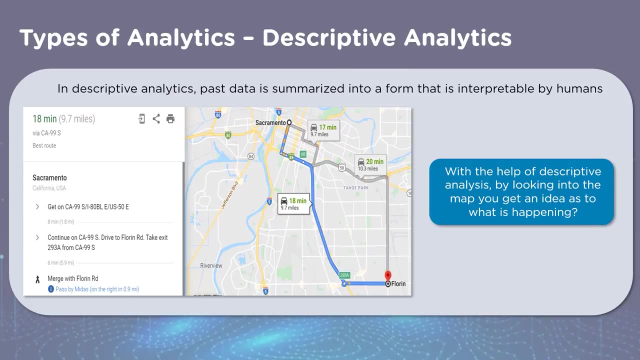 duration to travel, as well the distance. now let us understand what is descriptive analytics and why do we focus on this particular map example, as we understand the route map, the estimated duration, as well the distance to travel via the blue color route as well the gray color route, this is one. 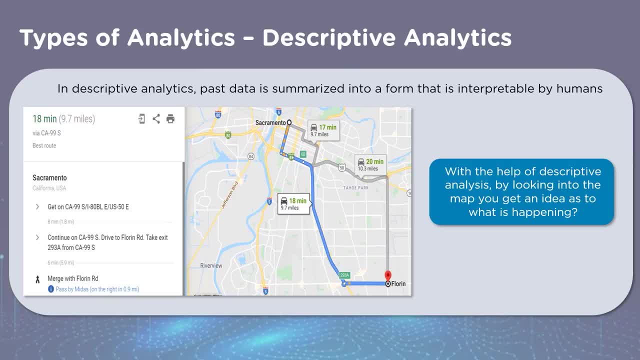 way of understanding descriptive analytics, as in what is happening. but there is another way of understanding descriptive analytics. that is by focusing on summarized past data, and this is a descriptive analytics. We see that what had happened in the previous year, Now let us focus on predictive. 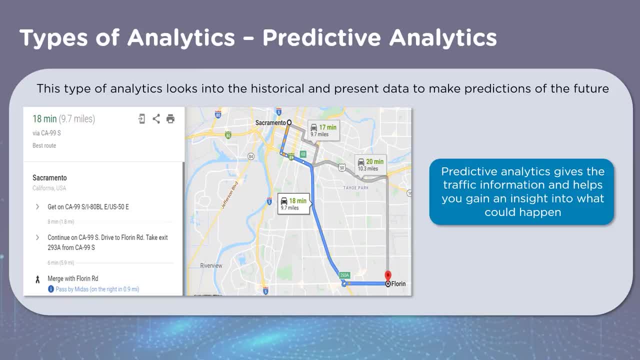 analytics. What is predictive analytics? This type of analytics looks into the historical and present data to make predictions of the future. What does this mean? So Google has already suggested the best route, which is the blue color route to travel from Sacramento to Florin, and the duration is 18. 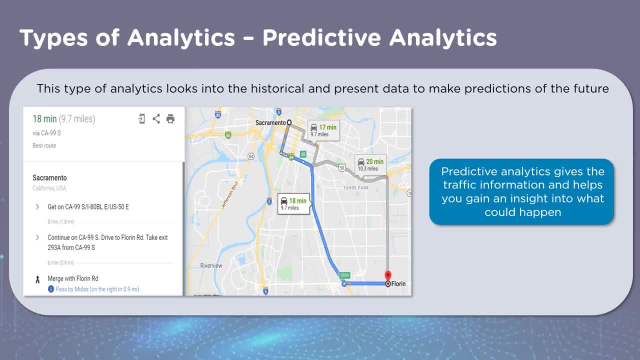 minutes and distance is 9.7 miles. Let's assume that Google map has already collected historical data of this particular route and, based on the available data, their model has predicted the best route and also the duration that will be taken. Now let us focus on prescriptive analytics. Prescriptive analytics describes the solution to a particular problem. 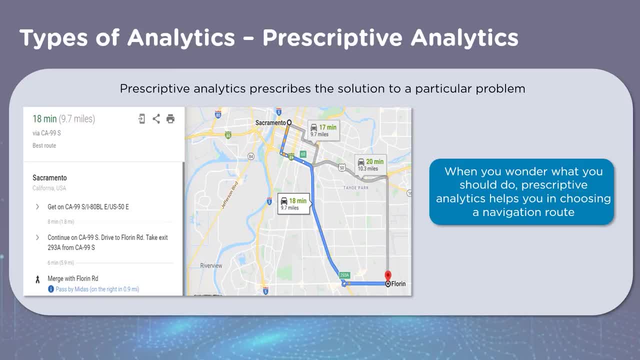 What was the problem in this case? on the predicted best route, Some predictions on the traffic congestions, and that's when Google map recommends the substitute routes Correct. Now these substitute routes are also prescribed by Google Map as a recommendation, So prescriptive analytics is nothing but a solution, and 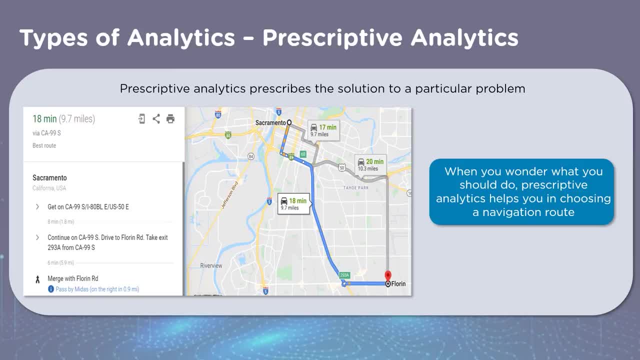 a recommendation provided for a problem. So in this case, we have the best route and we also have other substitute routes. So let's quickly summarize. Descriptive analytics is a both summarizing the past data or to see what is clearly moving on happening. for example, in the google map scenario. predictive analytics is about what would happen. 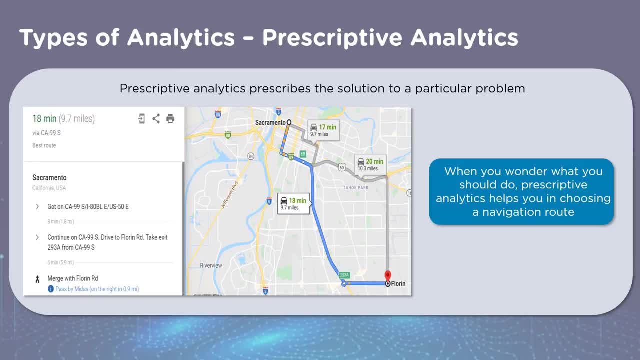 and prescriptive analytics is about prescribing the solution, the best solution and the recommended solutions. now let us refer back to mark's earlier scenario. mark, along with this team, identified the best model. they also did some testing and they got identified the best results and they also finalized on one particular model based on that particular model. now the results have to be. 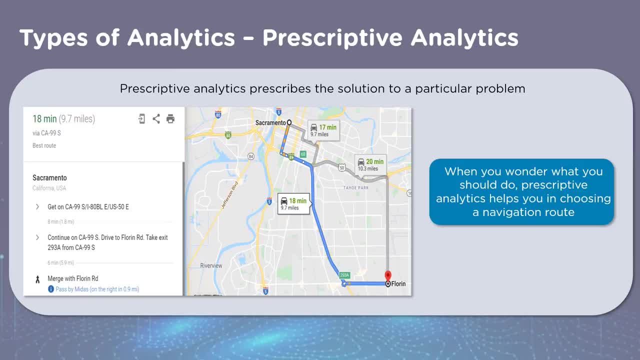 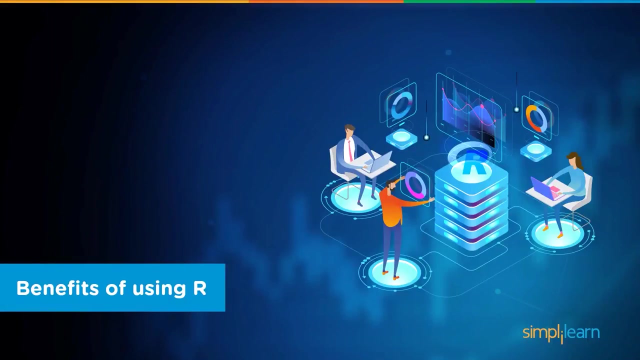 provided in such a way that they are the best results and also the recommendations correct, so it may not be just one single solution. it may be a solution with couple of other recommendations as well. so that is exactly what happens in the entire process of data analytics. i hope this has been clear so far. yes, okay, and now let us focus on benefits of using r. 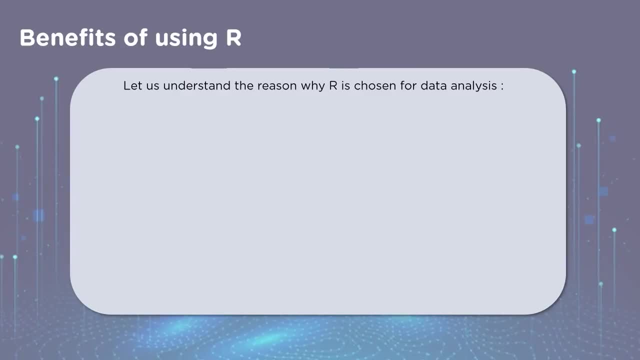 why do companies extensively use r for data analysis and why is it chosen? firstly, r is an open source programming language, which means that there is no license required to use r, and r does not require you to have a coding experience, which means that a non-technical person 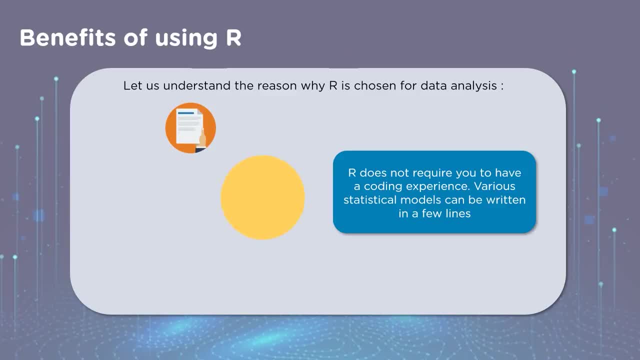 in your team can also learn r very easily and start coding or building models in few lines of codes. r can also be used with other programming languages such as java, c, plus, plus and python, and the integration of r with other programming tools or bi tools is very simple and easy. 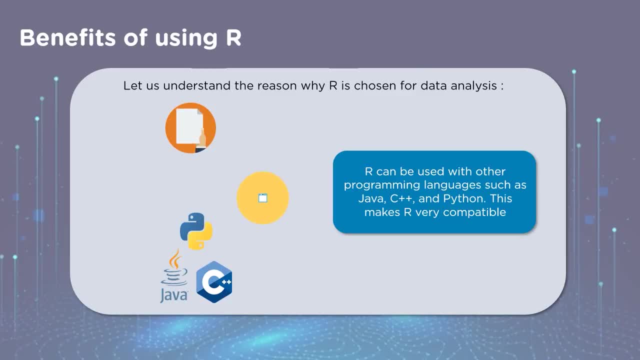 and various statistical models are readily available in r, which also means that there are plenty of inbuilt libraries and packages already available, and reporting the results of an analysis becomes easier by using these inbuilt packages and for creation of these models in just simple, few lines code. with this understanding of the benefits of fusing r, 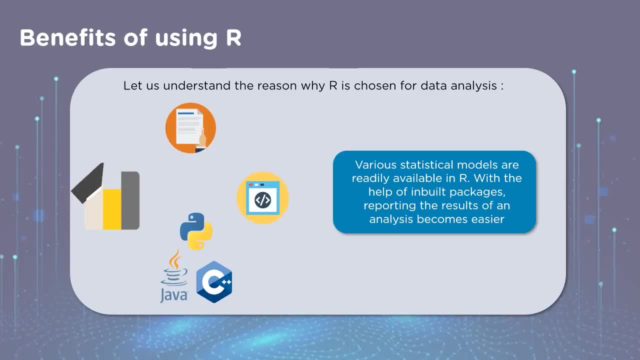 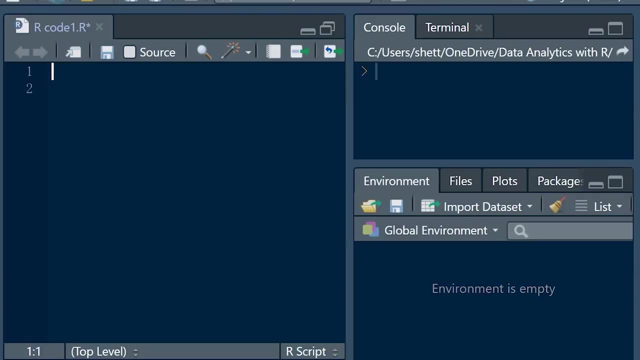 let us quickly hop on to our studio and start performing the hands-on exercises for data analysis. for this exercise, we will use a data set named as demographics, which is in a dot csv file type. firstly, let us load the data set to our studio and we will locate this in a variable. 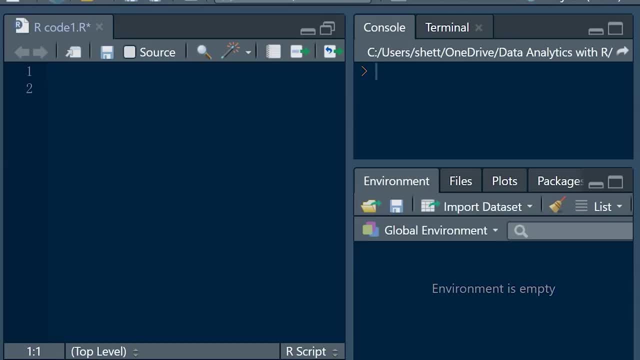 named as demo. we also refer to this as a data frame, and now you will notice that a variable is created in an environment section, which is in the bottom right hand side of the r studio window, and this particular variable comprises of 510 observations or records with 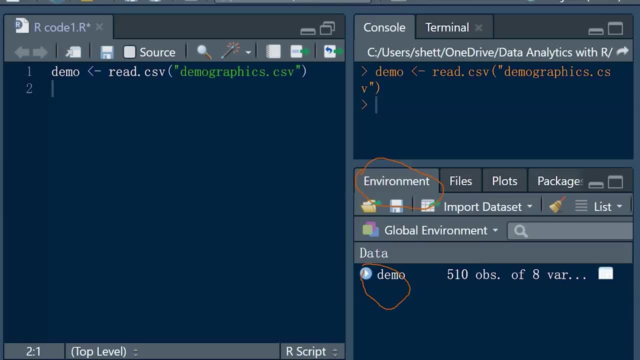 eight variables. let us simply expand this particular data frame and have a quick check on the data structure and understand the data types. this particular data frame includes variables such as age, marital income- the unit of income is dollar per day day- education levels, the car price, car category with several levels, gender and retired. 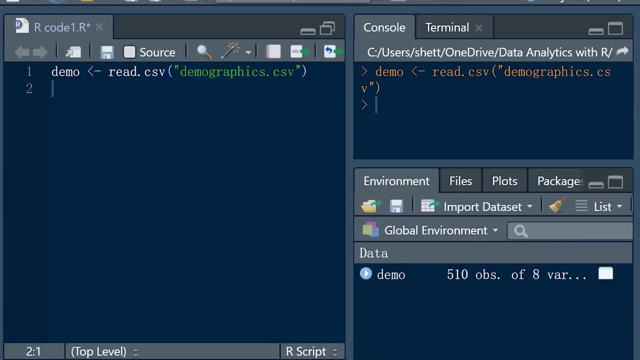 status. Now let us view the top six records of this particular data set. For this, let's simply type head of demo and the result is now visible in the console section. If you're interested to view all the records, then simply type view of demo and this new. 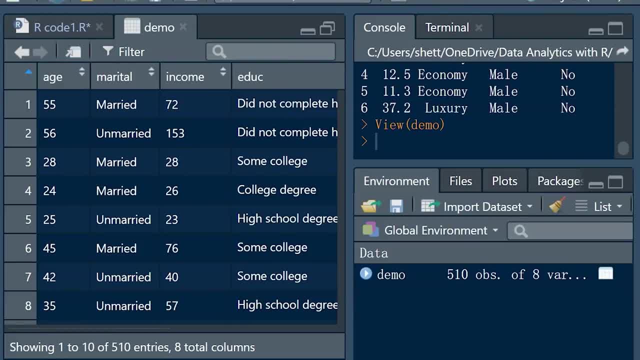 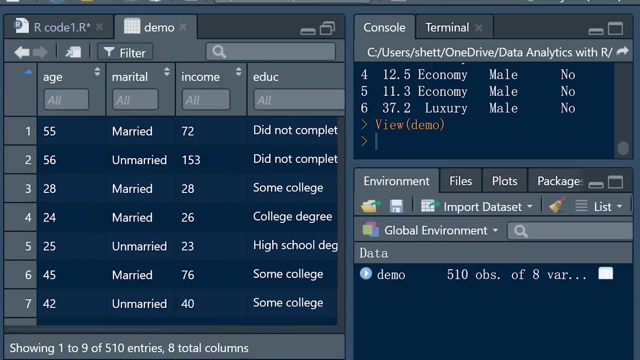 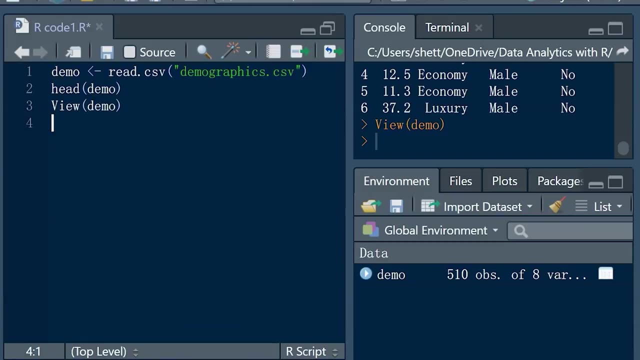 window will show you every single record that is being loaded to our studio. You may also simply apply the filters and the filter section here on individual categorical variables. Now that we have loaded the data set and also viewed individual records, let us focus on creating subsets of records by applying filters on individual variables or multiple variables. 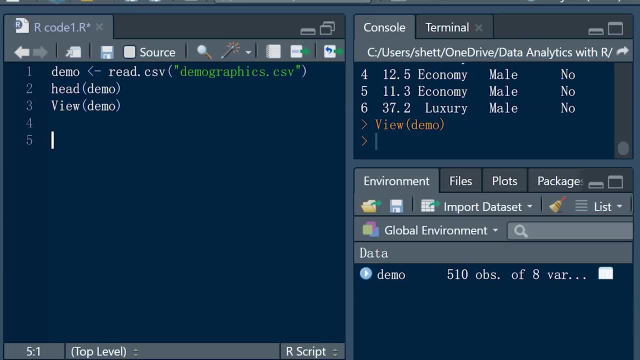 So, firstly, let us apply filter on gender. We will only retrieve the records where gender is equal to female and we will locate these records in a variable named as demo2.. As you notice, now in the environment section, the second variable is also created, that is: 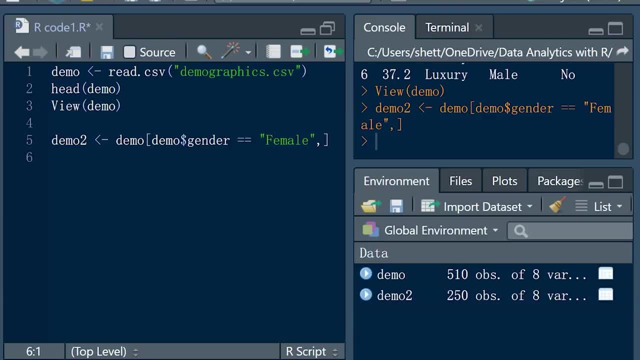 demo, and this now is comprising of 250 observation, which means the records are filtered down to only gender: female. Next, let us see how to apply a filter on income variable. Let us only retrieve the records where income is greater than 100.. Okay, 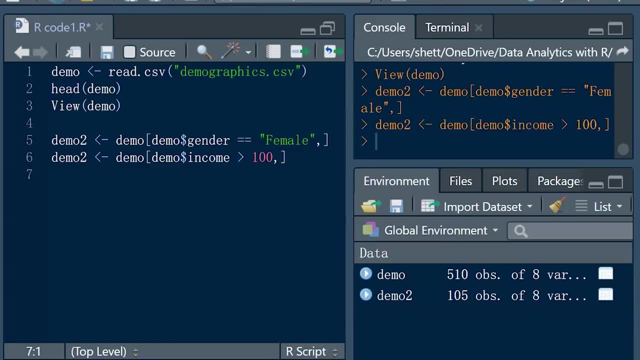 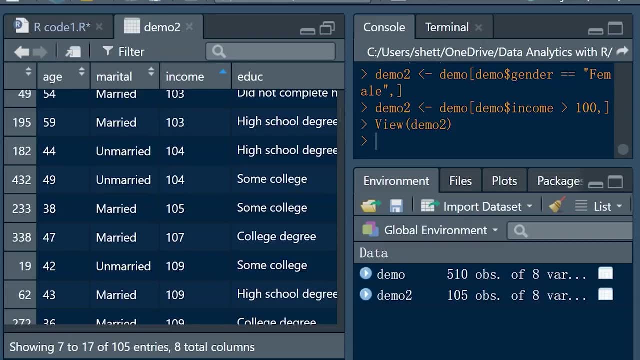 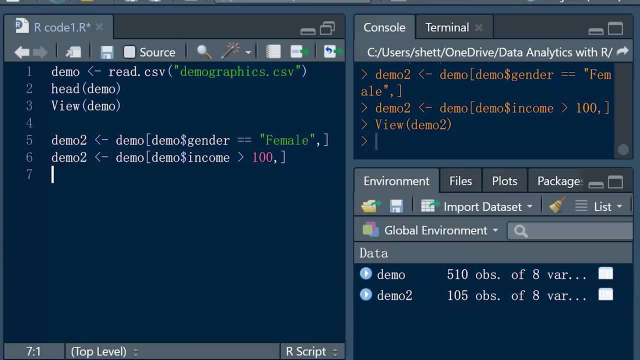 Let's view the result As we see here. all the records include income greater than 100.. Now let us modify this query and we will ensure that the retrieved records includes income greater than 100 and also specific variables are returned. Let's say, we only want to have 100. 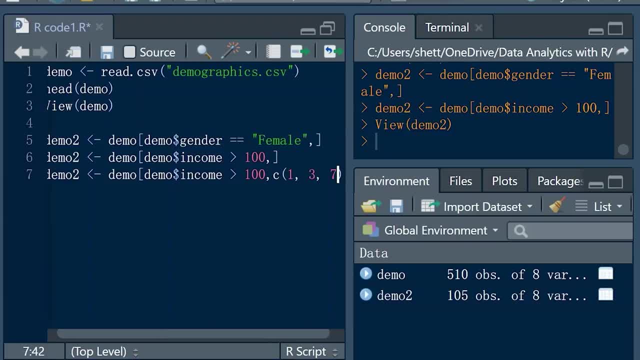 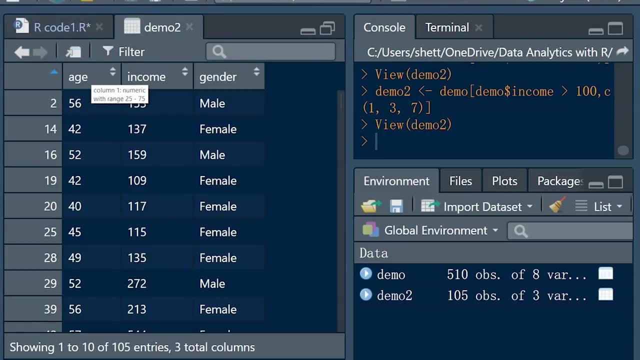 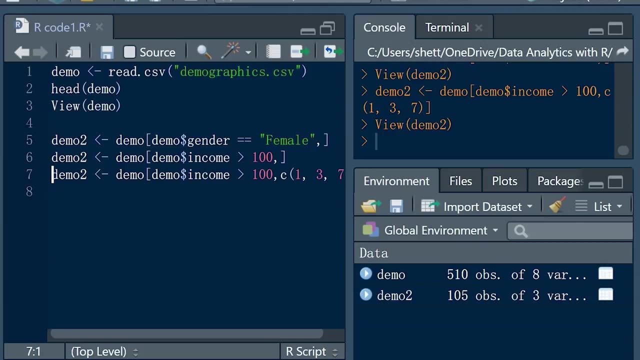 Let's say we only want to have the first variable, third variable and the seventh variable returned. as the result, Let's have a quick check. So we only have the first, third and the seventh variable returned. How about we only exclude the variable 6 to 8.. 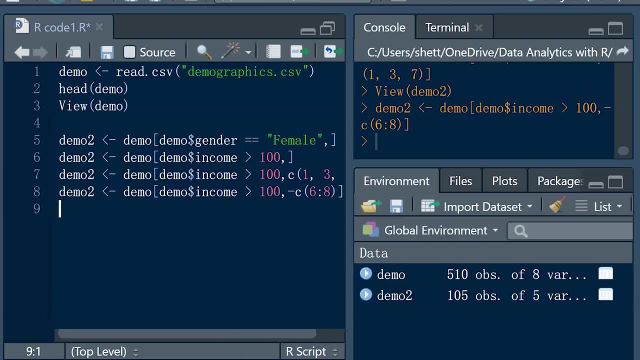 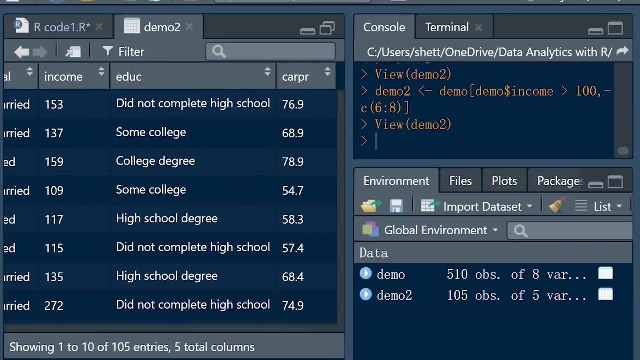 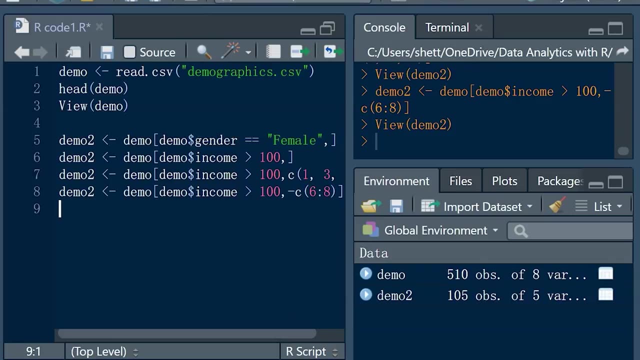 For this we include a prefix of minus sign. Okay, And now let us see what is the result. We have the variables from first to the fifth variable. however, we don't have sixth, seventh and eighth variable. I hope it's clear so far. 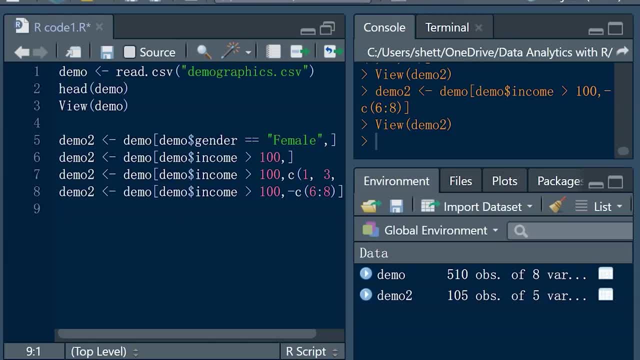 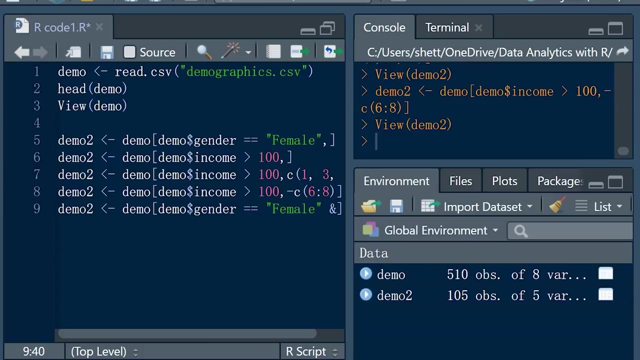 Yes, Alright, Now let us see how can we apply condition by including both the variables, that is, gender and income, and then we will filter the record and create a subset of data. So we will have the first value, which is Уnit, which is a lovely little value that we 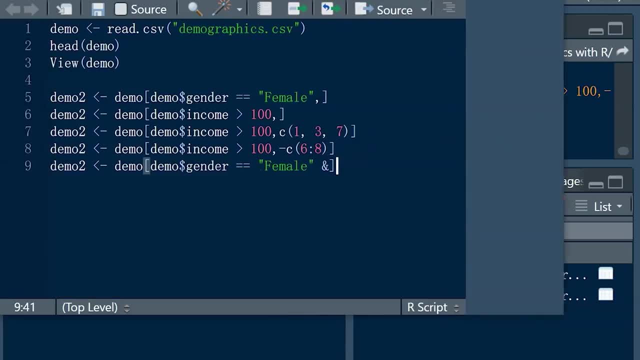 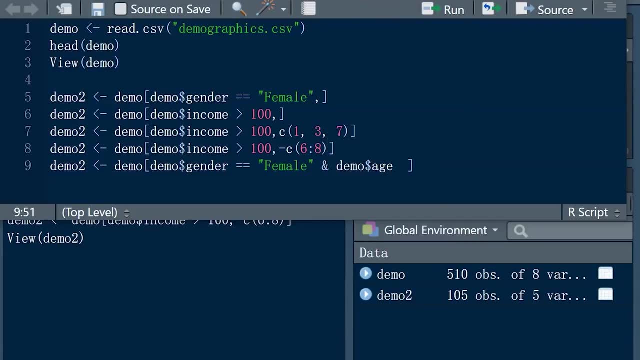 can drag it to the top of the table. So if we click on it and go to the next screen, we will see that we have Unit with the first value in the second row, And then let us add another value, which is Unit. 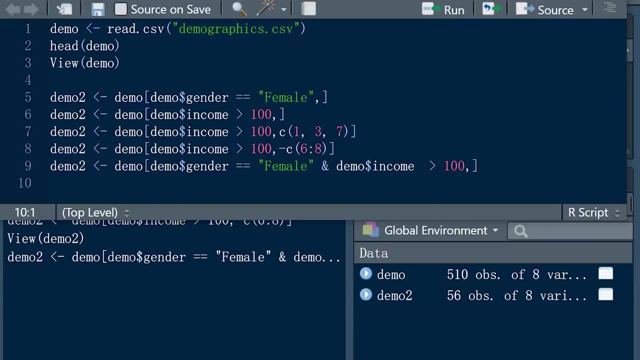 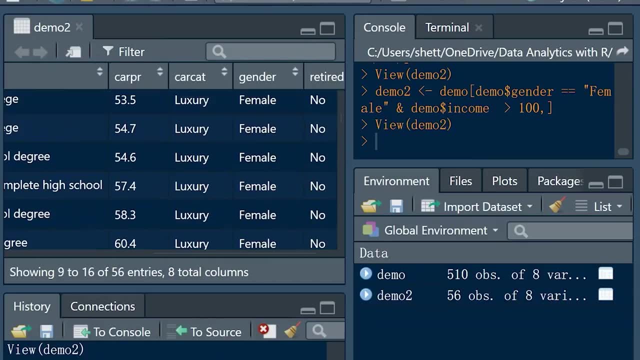 So a little bit of change required here. We have the first value there. We have a second value here. Let us apply it to the first cow view. the result Income is greater than 100 and the gender is only female. This 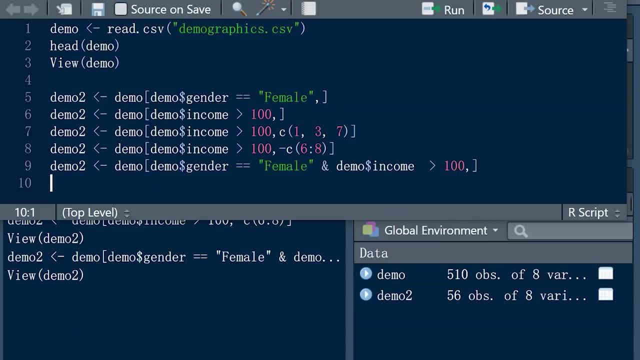 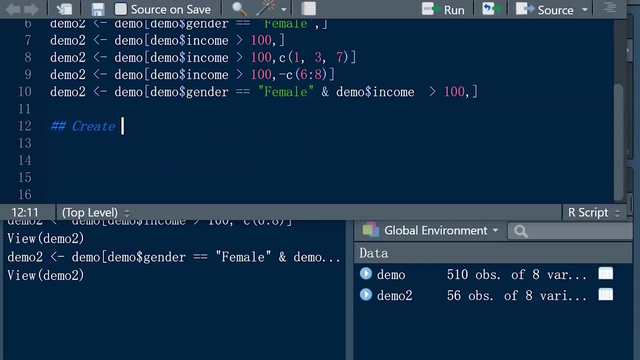 is one way of creating subsets. However, now let us see how to use the subset command and create the subset. Let us create a subset of records by applying filter on marital status and age. We will only retrieve records where marital status is equal to married and age is greater than. 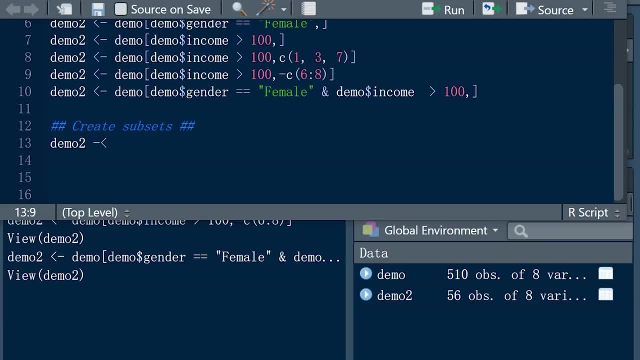 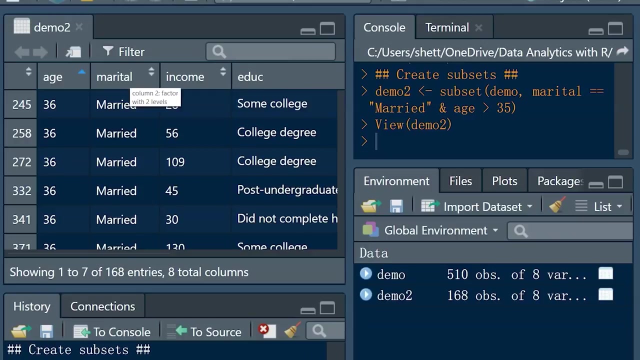 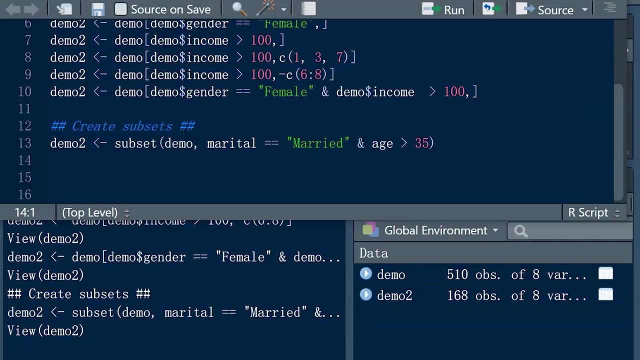 35.. Let us create a subset of records by applying filter on marital status and age. We will. Let's now view the result. So here we have the age greater than 35 and marital status is married. Let's use the same code and this time we will retrieve selected variables. 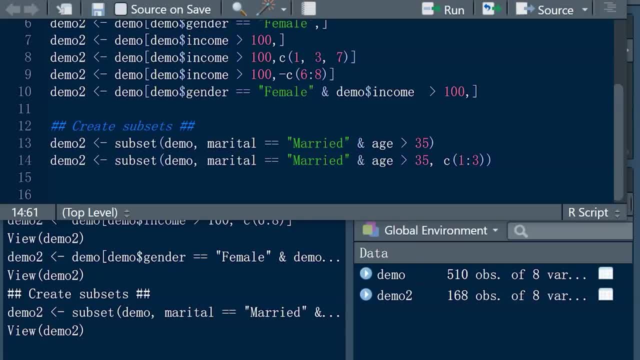 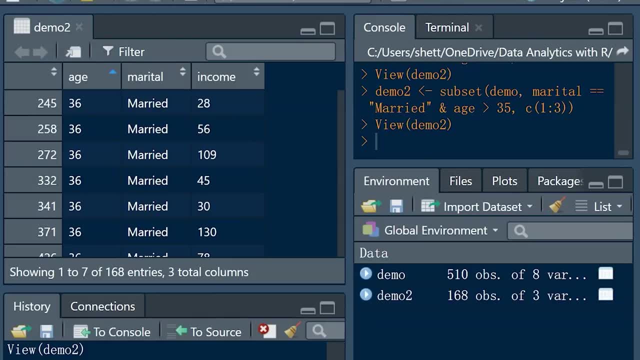 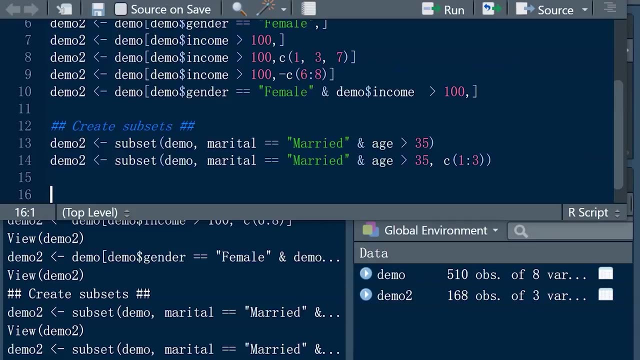 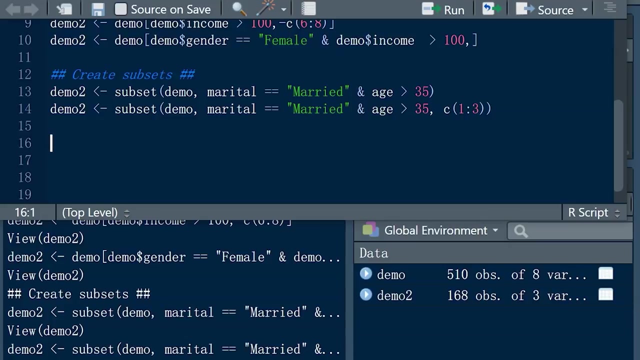 Let's say variables ranging from 1 to 3.. Let's have a quick check. So there are three variables: age is greater than 35 and marital status is married. Now let us see how to structure the data by sorting the data frame in ascending and descending. 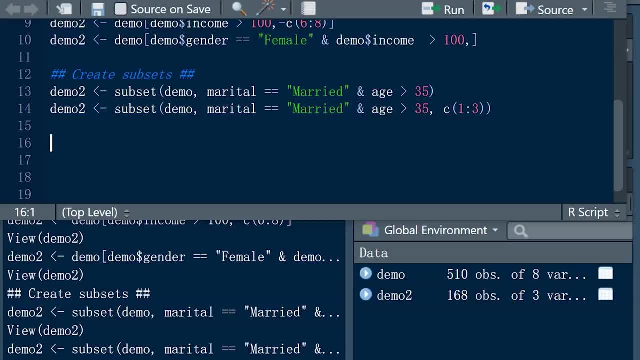 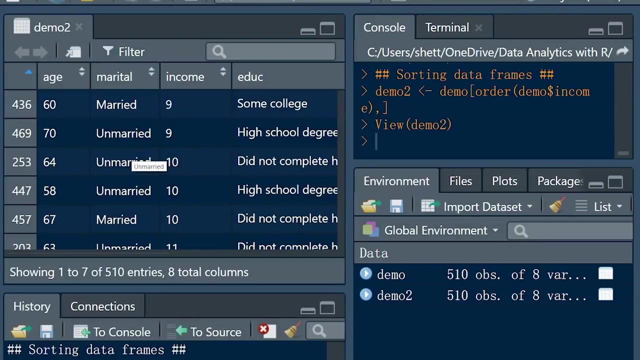 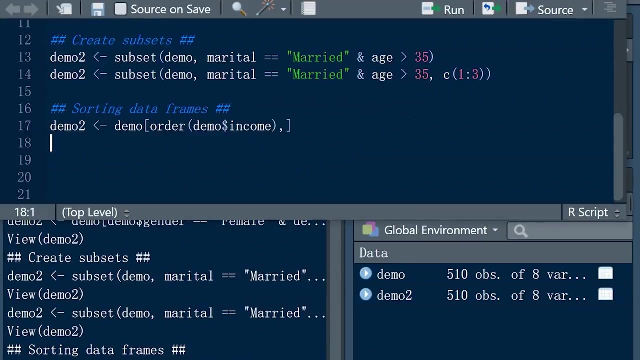 order. We will apply this order function on the variable income. Firstly, let us see how to order income variable in ascending order. Let's do a quick check And here we have income in ascending order. Now let's see how to modify this. 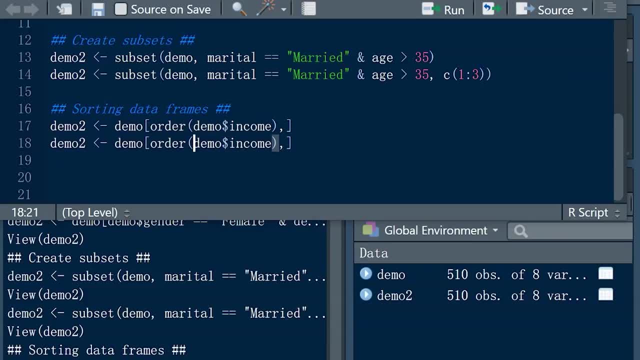 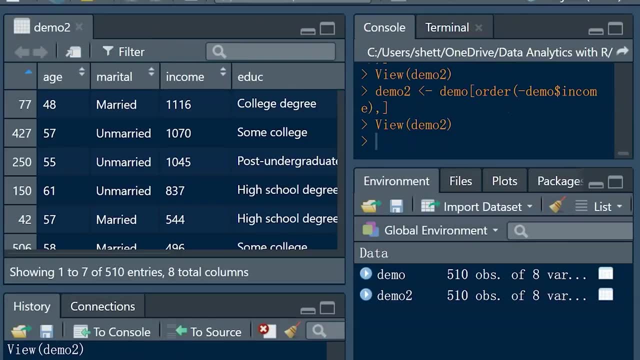 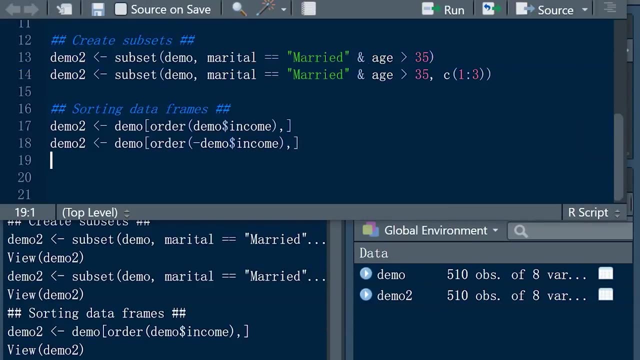 Okay, Let's use the same code and view the records with income in descending order. So we have now the income in descending order. How about include two variables and sort the variables accordingly? Firstly, we will sort the records by ordering income and age in ascending order. 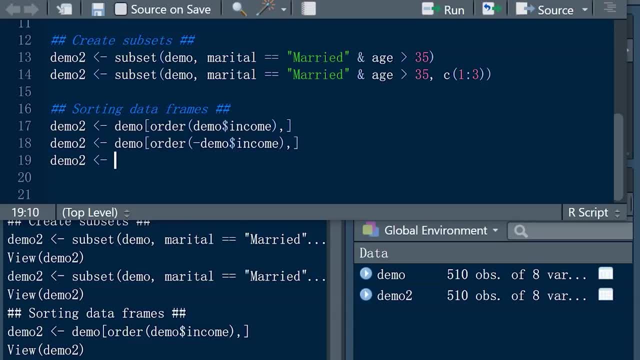 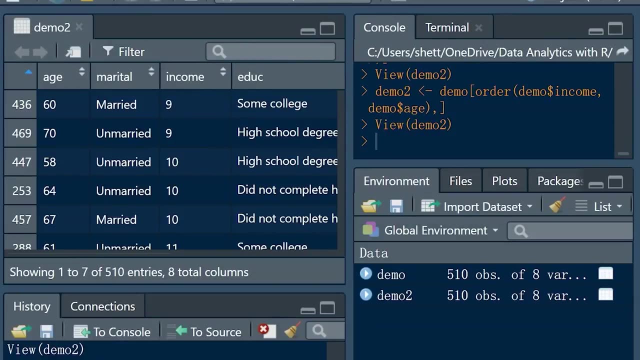 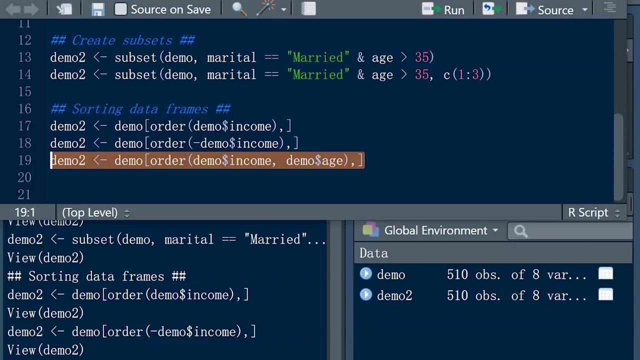 Let's quickly view the result. We have income in ascending and age as well in ascending. Let's now modify this code. This time we will order income in ascending order, Income in descending and age in ascending order. Let us view the result. 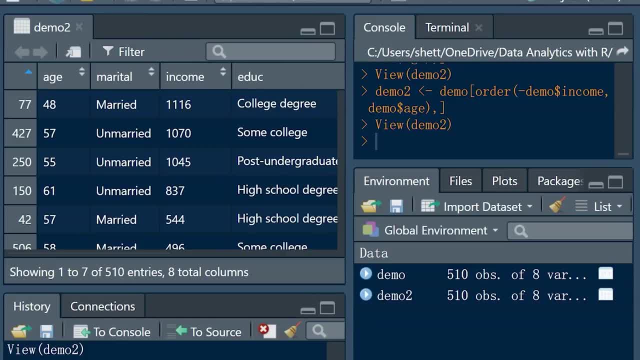 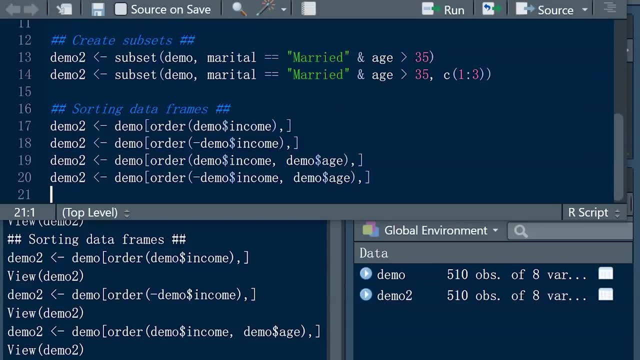 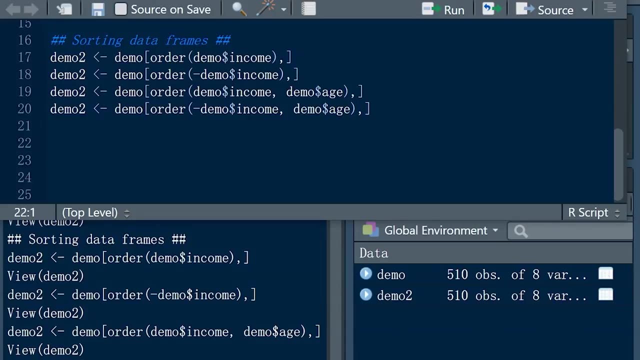 So the income is in descending and age is in ascending order, So hope this is clear on how to sort the data frame: by ascending and descending order per variable or by using multiple variables. With this we will focus on learning statistical analysis, How to perform data analysis. 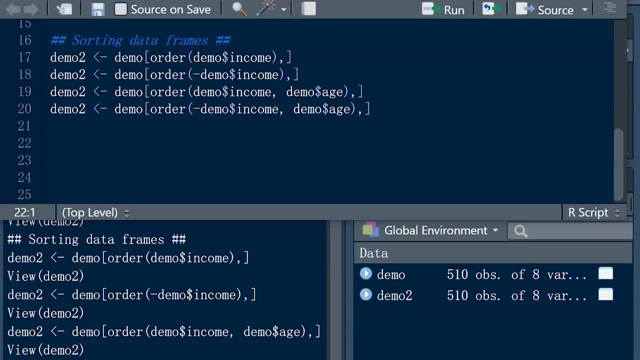 How to perform statistical analysis on individual variable or multiple variable. Let's start by understanding the data distribution of variable income, So that we identify what is the minimum value of income, What is the maximum, What is the range, What is median, What is the mean? 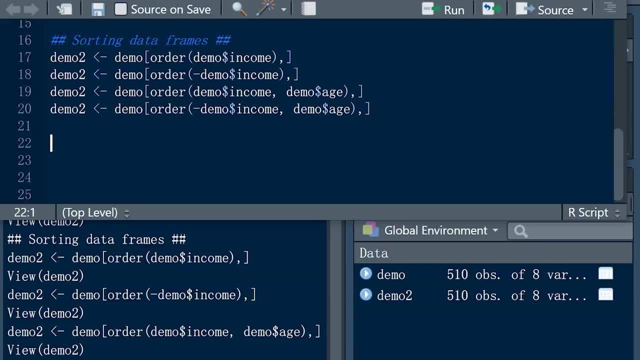 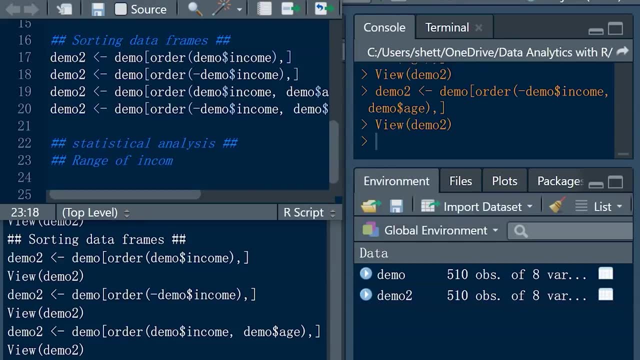 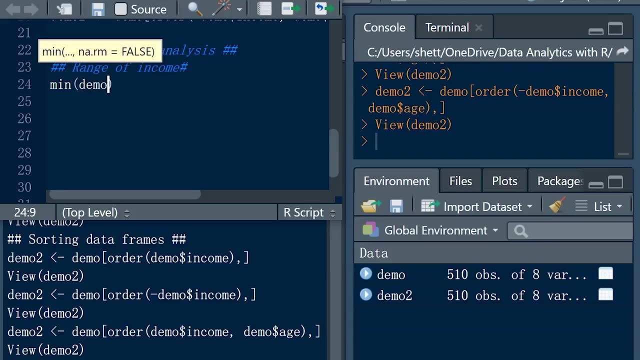 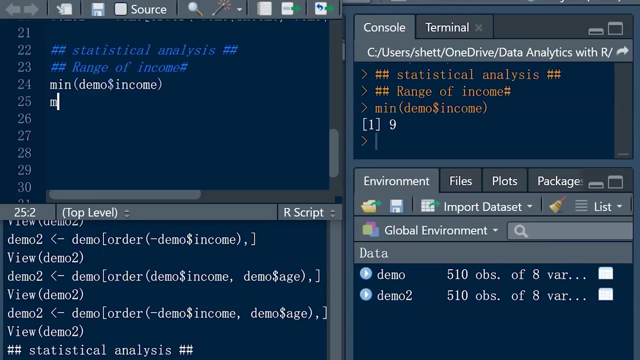 And we will also focus on the quantile distribution, Which is also analyzed in a box plot, For example class. what is the minimum value of income? So in a table class we will write the value of income as minus to the minimum. What is the minimum values value in the variable income? 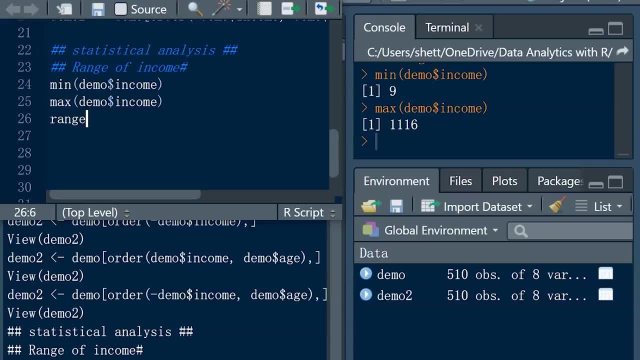 What is the minimum value of income? So is this the range in this table here? Then we will start by understanding what is the minimum value value of income, Given that it is 9 washing minutes. for the math it is 9.. Where is the range? 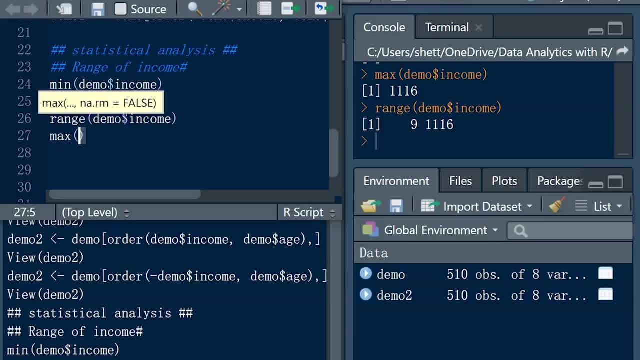 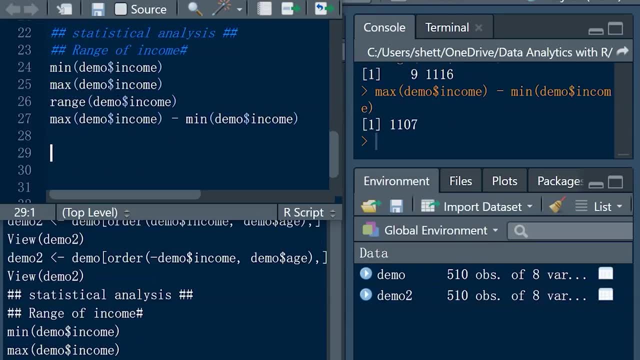 Let us now define the value of debdull. What is thebest? mate value, the maximum value? how about the difference of maximum and the minimum? now let us focus on other summaries of data distribution for this variable income. let's identify what is the mean. 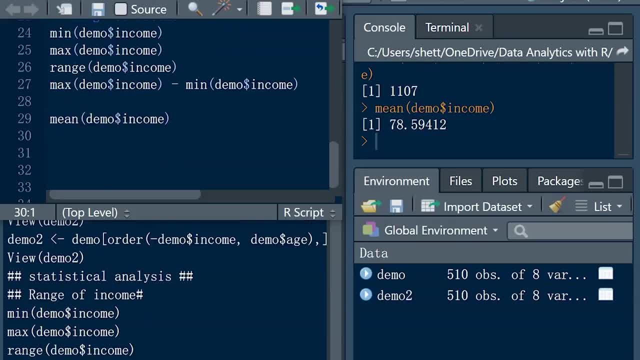 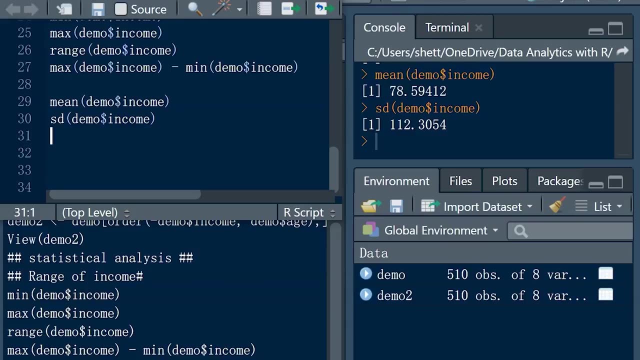 value of income. the mean is 78. let's also understand what is the standard deviation. all right, so the standard deviation is 112 dollar. let us see what is the variance. the variance should be larger than the standard deviation. now let's see what is the median absolute deviation. 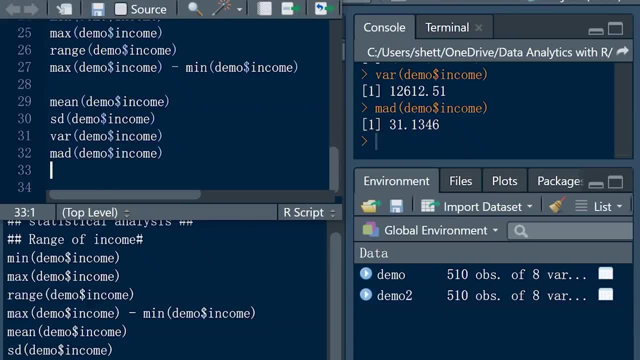 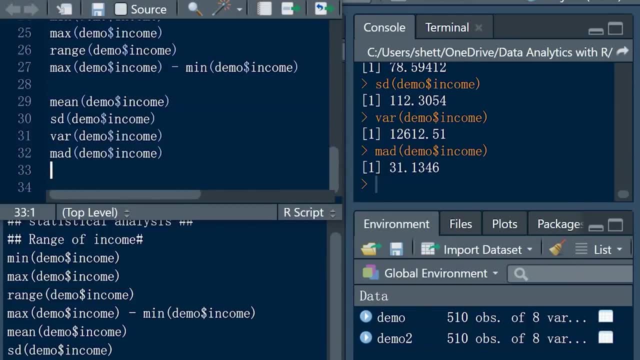 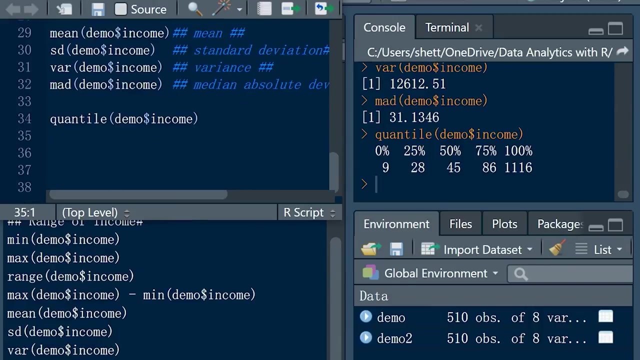 as you notice here, the median absolute deviation value is lower than standard deviation. why do we make this comparison? from this, it is evident that median absolute deviation is robust to outliers and standard deviation is sensitive to outliers and also to the change in the mean value. now let us understand the quantile distribution. this is the same analysis that is visualized in a 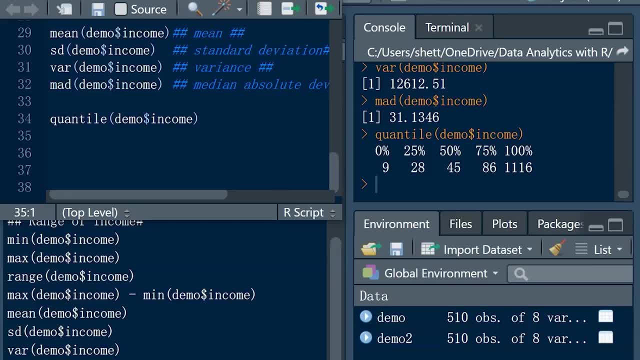 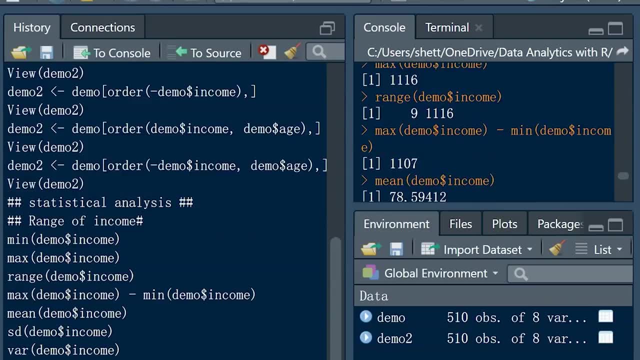 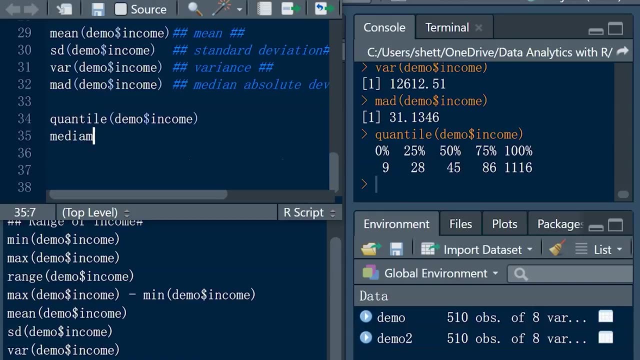 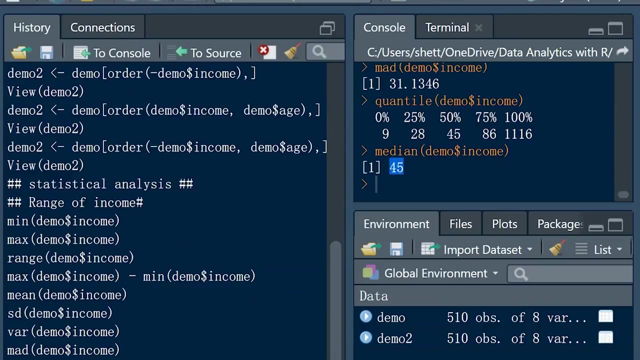 box plot ranging from zero percent to hundred percent, identifying the individual data points, and we can also refer and compare this to the min, the max and the median values. let us quickly see what is the median value of income. as you notice here, the median is 45 as well. the 50th percent of quantile is 45, which means zero. 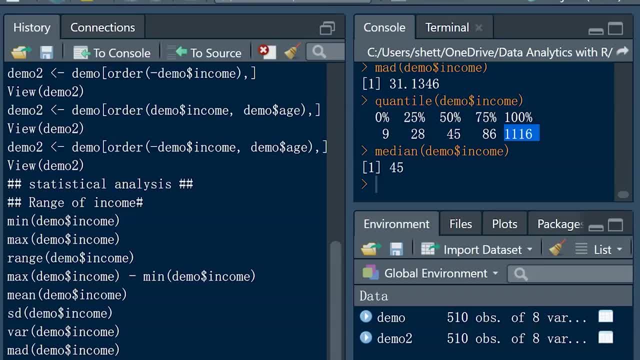 percent is minimum and hundred percent is the maximum value. now, if your question is: what is 25 and 75 percent? this is again used for identifying the range of interquartile. the interquartile range is nothing but the difference of 75 percent minus the 25 percent. 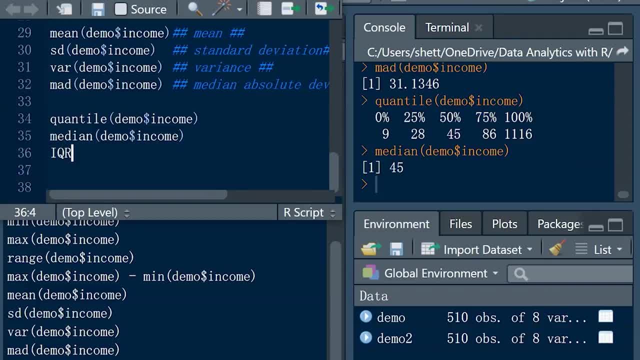 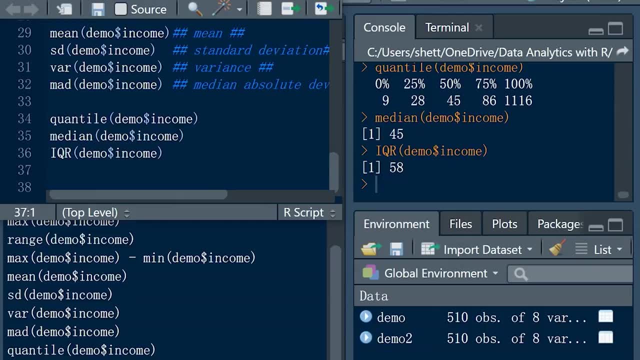 let's quickly see what is the iqr of income. the iqr of income is 58. let us do a quick check: 75 percent of quantile is 86 and 25 percent of quantile is 28 and the value is 58, which is equal to the iqr result. 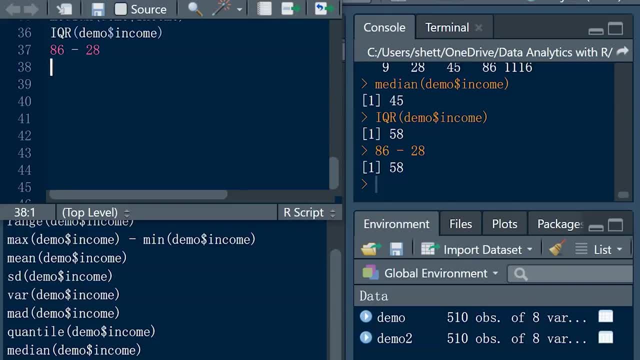 now that we have focused on the statistical analysis of the individual variables, data distribution, let us focus on the data visualization. in this we will have a pictorial representation of analysis to identify the outliers, to see what is the minimum and where do we see the data densely populated and how is it scattered, etc. we will begin with creating a histogram. 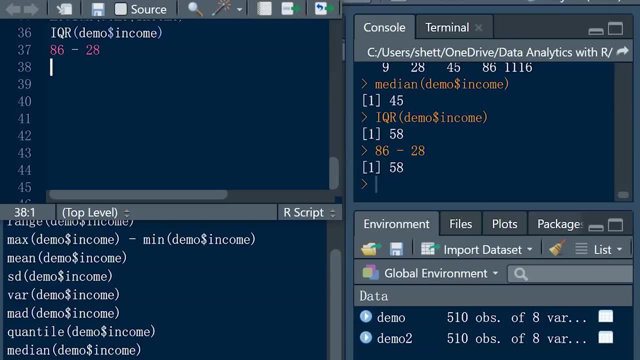 now histogram can be used for your computer univariate analysis, which means in this scenario we will consider income variable and we will see how the count of income ranges gets distributed in a histogram. for this we will have to install a package called as ggplot2 and also call this library ggplot. let us install the package. 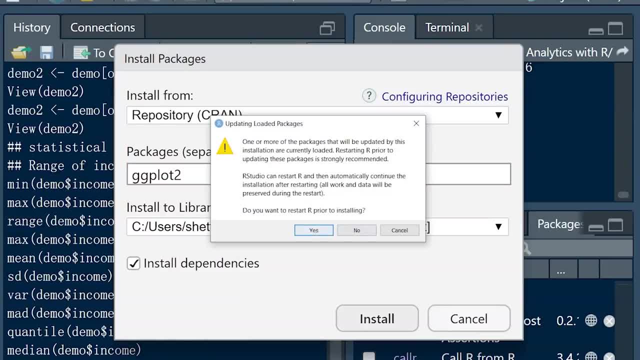 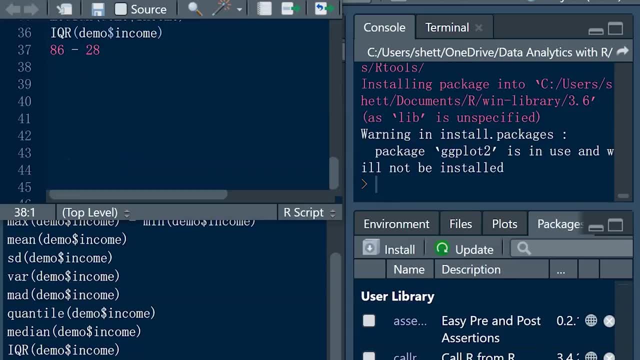 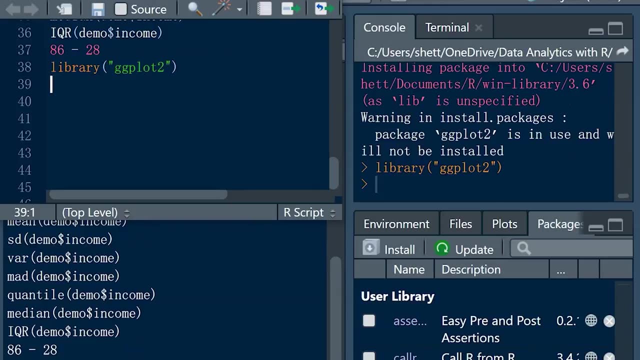 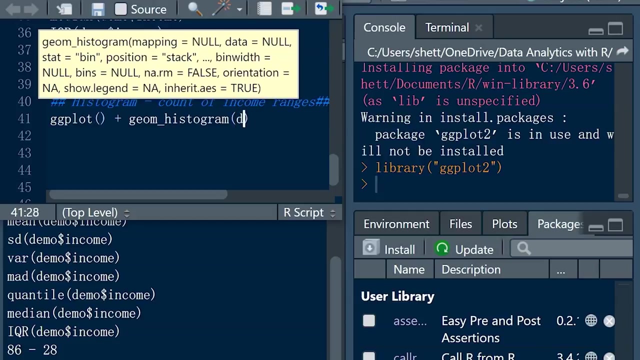 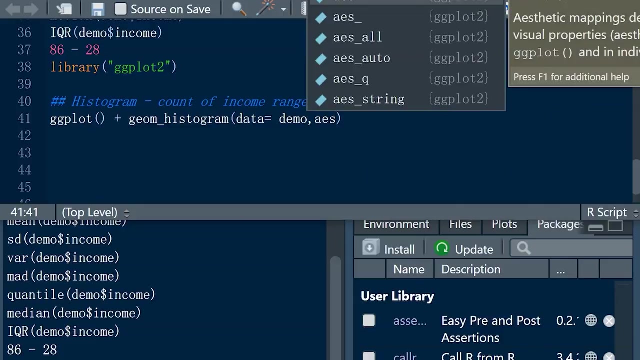 ggplot. now let us call the library all right, and we are ready now to begin with visualization. for this we will use the geometric object histogram on the data demo data frame. let me expand this window so that the code is visible and also use an aesthetic mapping for variable income. this will be helpful for filling colors. 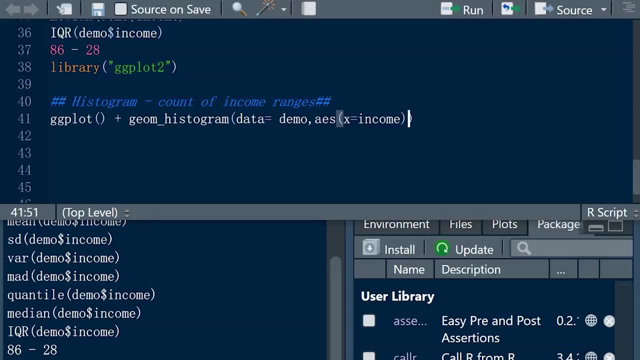 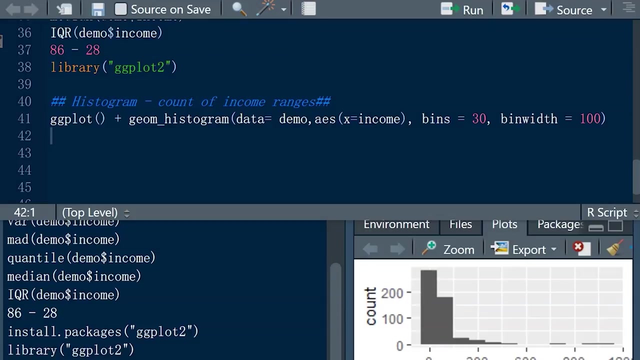 or filtrations and so on, etc. and only include 30 bins with individual bin size width of 100, which means there will be hundred incomes in individual bins. let's quickly look at the distribution of this histogram. as you notice, there are couple of outliers. the counts of these income range are very limited. however, we see the densely. 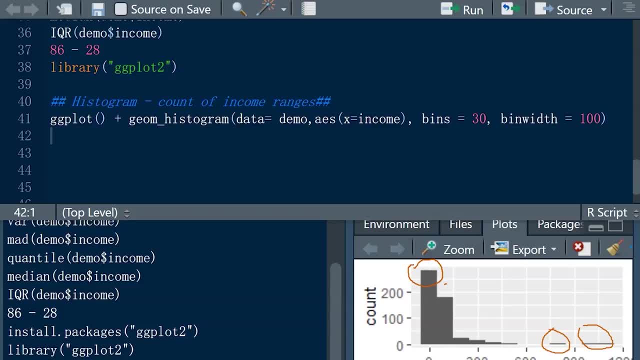 populated income ranges with higher counts, between 0 to 200 dollars per day. this is also a way to identify and segment the customers based on their income ranges. now let us see how to change the color of this histogram and also the border of the histogram. for this we 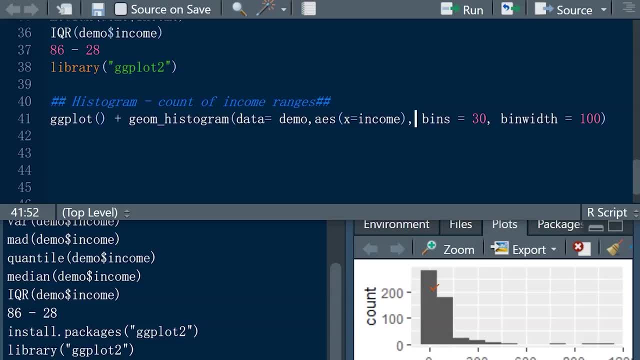 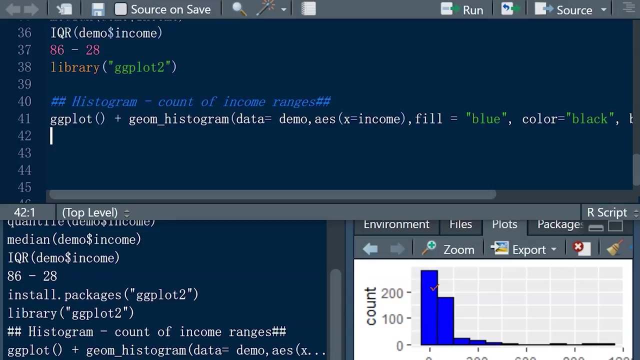 will include some additional options, such as fill, fill with blue color and the border color is black. now, as you notice, here, the executed code is provides us the histogram with blue color bars and black color borderlines. now we will focus on creating a facet grid. facet grid is also an aesthetic. 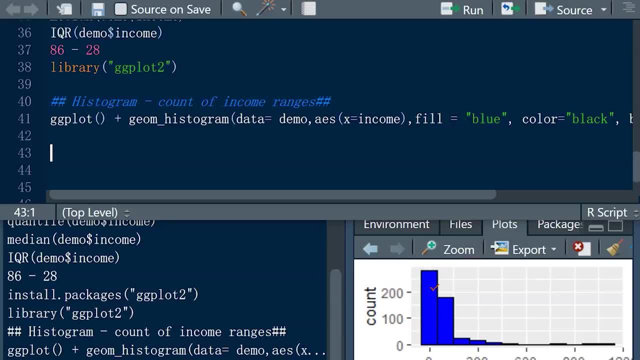 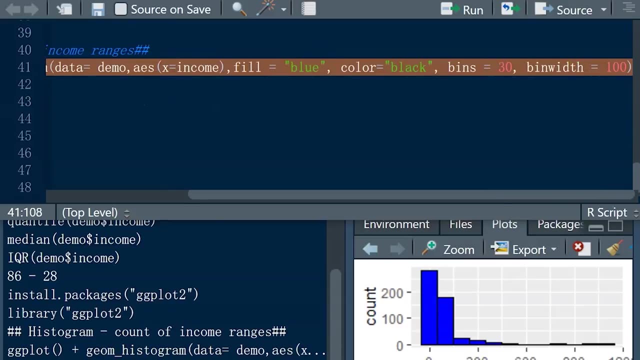 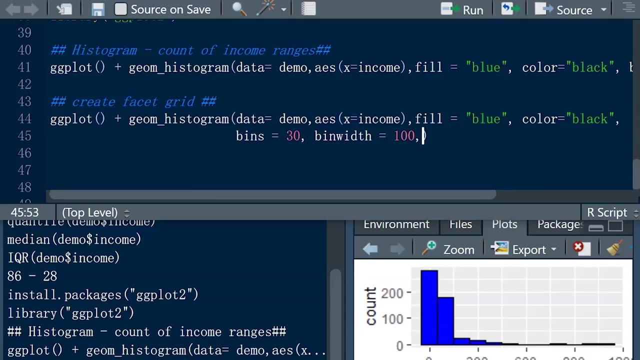 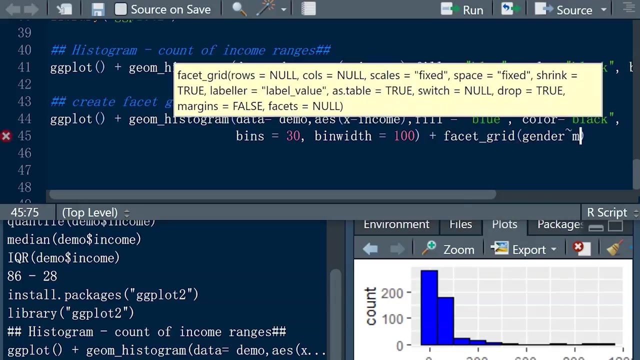 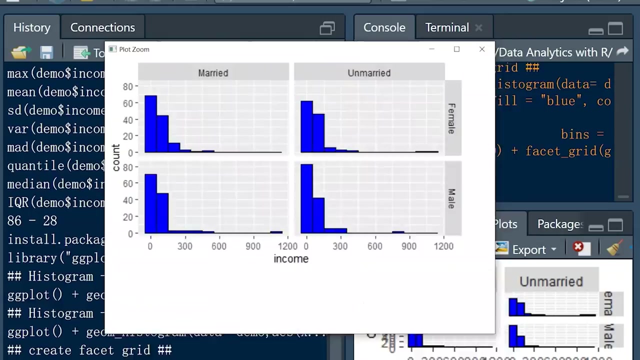 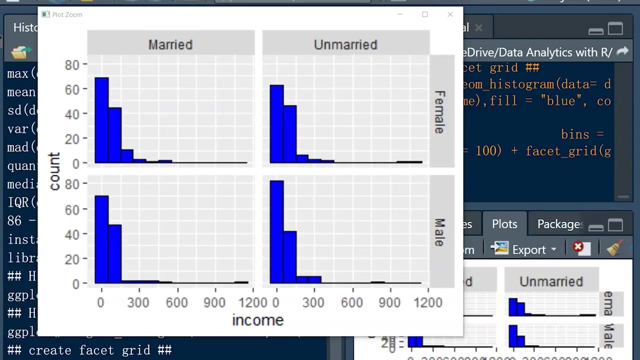 mapping object. we will see how to enable the multiple histograms across the marital status and the genders so that we identify how the income is distributed for individual marital status as well. the genders are nothing here. here in the data distribution, female unmarried drawing higher income and male unmarried and. 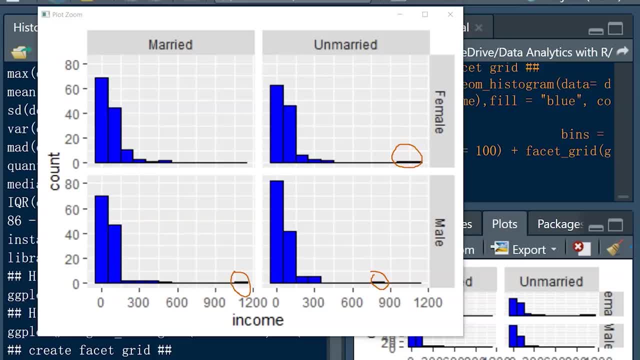 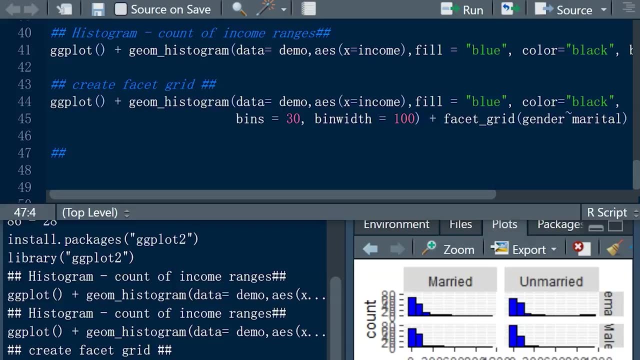 married also drawing higher income as compared to the females, whereas if you notice that the female, unmarried, is drawing much higher income than the male, this may also be very much related to the age. now let us see how to create a stacked histogram. when i say a stacked histogram, i mean 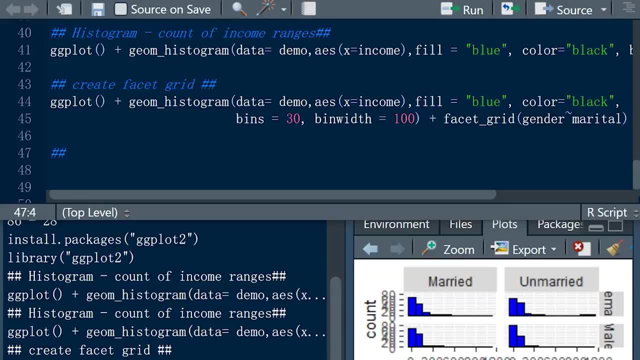 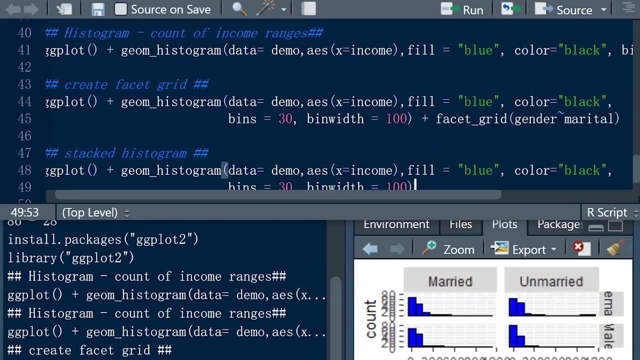 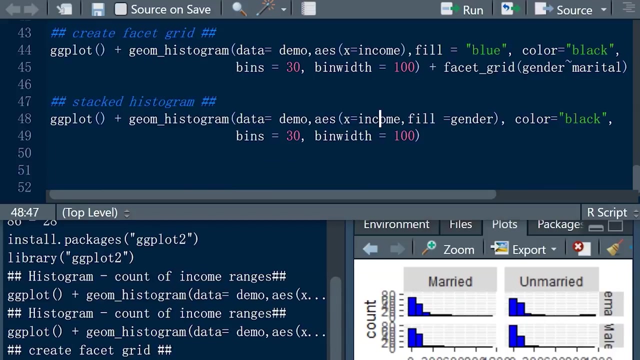 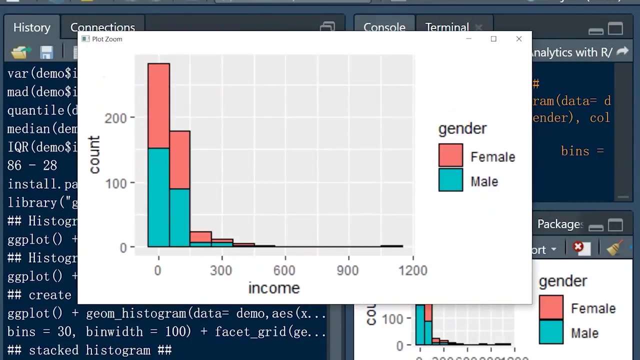 instead of filling the color, we will fill the gender, so that there is a stack within the histogram. so, as you notice, here i have made couple of changes. i have included fill equal to gender within the aesthetic mapping. now let us look at this histogram. as you see, here the gender is filled in the histogram, hence we have stacked distribution. 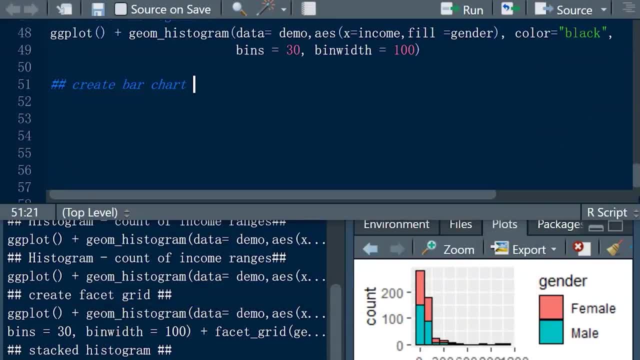 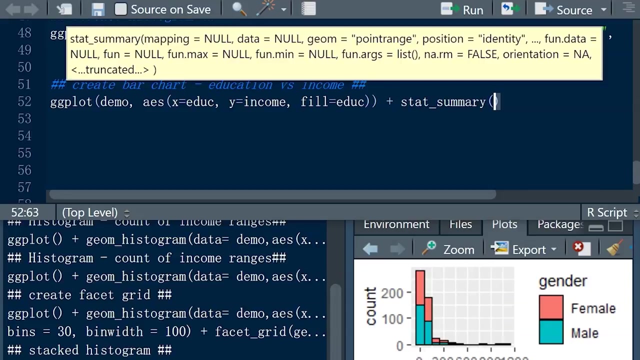 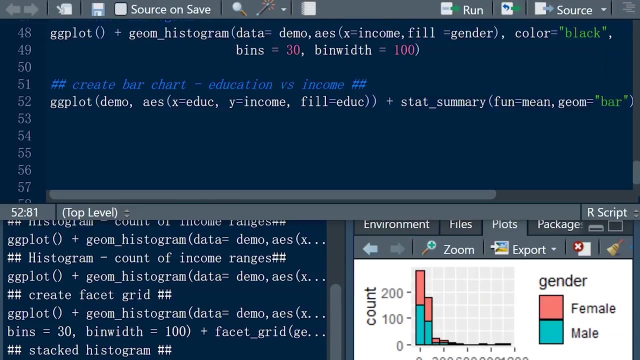 of female and the male. now let us focus on creating a bar chart with education versus income where we can identify the education levels and the income ranges for these education levels. as you notice, here we are going to create a visualization where we have the aggregation in form of mean and the geometric object used to show the 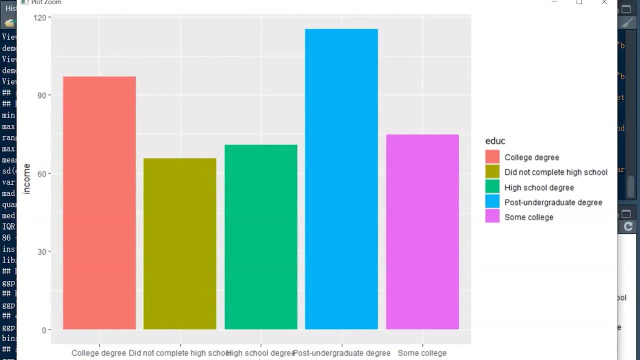 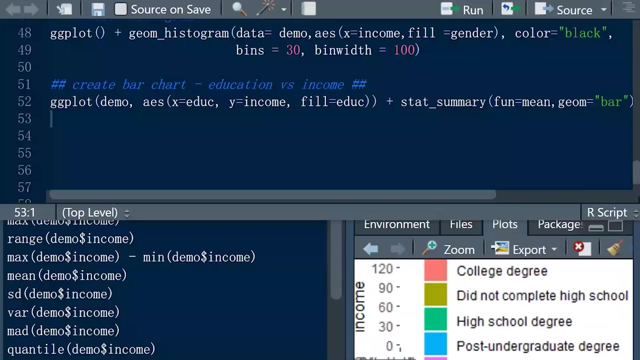 here is bar plot. now let's zoom this view and understand which education level have higher average income. so, as we see here, the blue color bar is the post undergraduate degree, which means this education level draws higher average income as compared to other education levels. now let's create a histogram where we will see car price and the number of cars for individual. 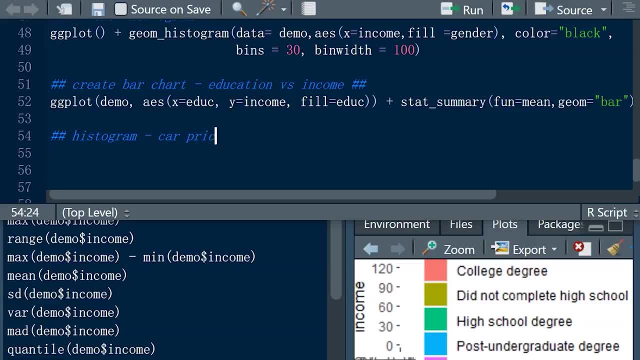 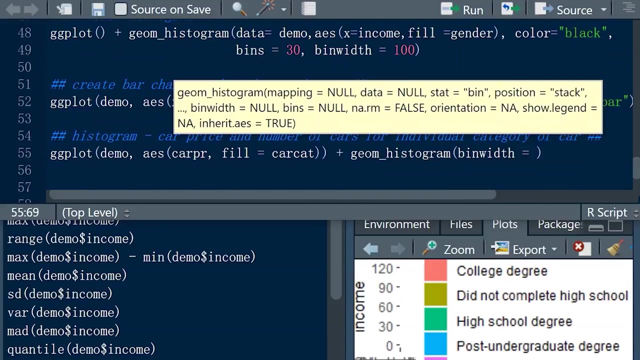 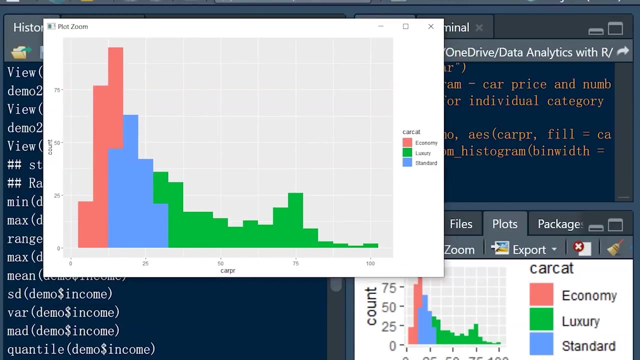 category. let's look at this visualization. this visualization provides us some interesting insight just by looking at the distribution of the car prices and the counts of the cars at the car category. economy and even the luxury- luxury car category of car price is pretty much distributed, whereas economy car category is tensed. 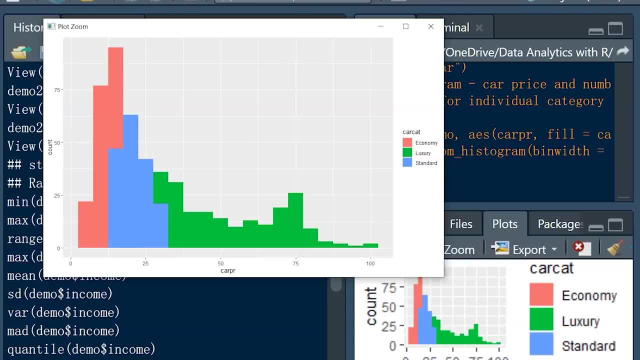 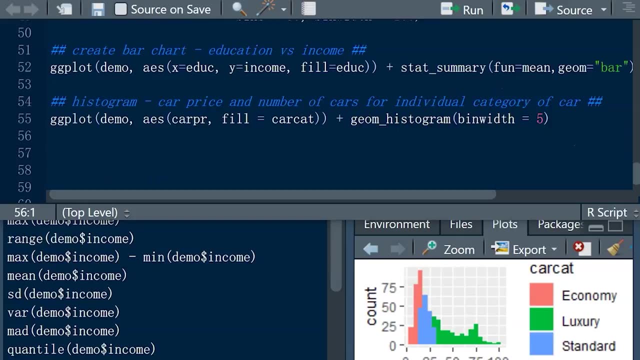 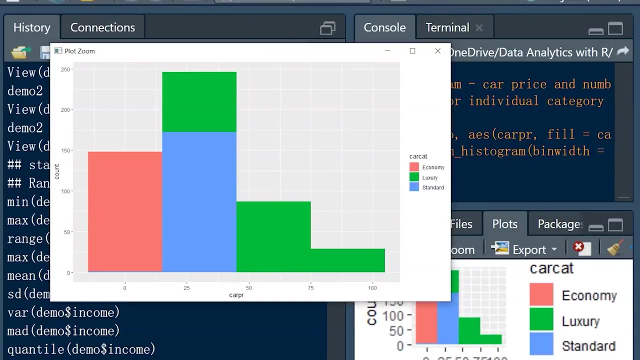 which means that we could also look back into the income and age variables and try to figure out further, more insights and then segment the customers for further targeting of these customers. now, what happens if we simply change this bin width to 30.. as you observe here, changing the bin width or increasing the bin width will also reduce. 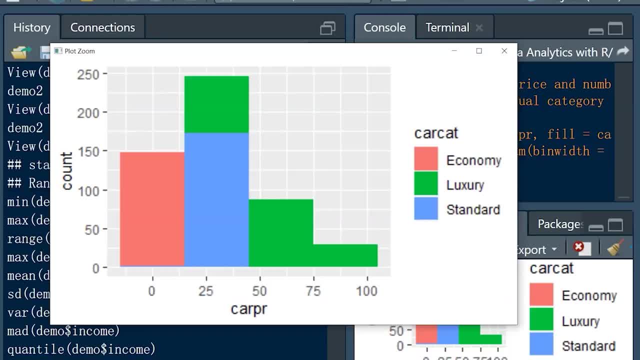 the number of bins. now we only have four bins here and the car category is filled. that is what we have enabled within the aesthetic mapping and we see some more interesting inside. as you look at the standard and the luxury car category, the car prices are pretty much overlapping for the car category. 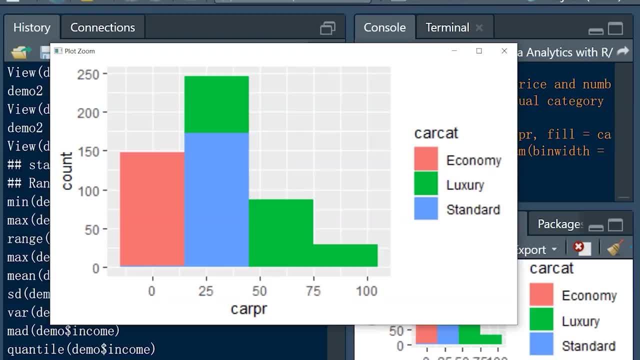 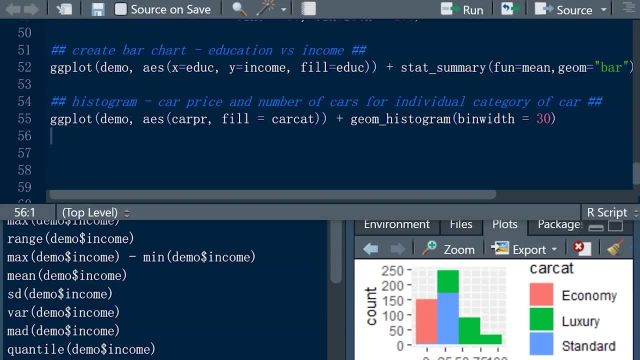 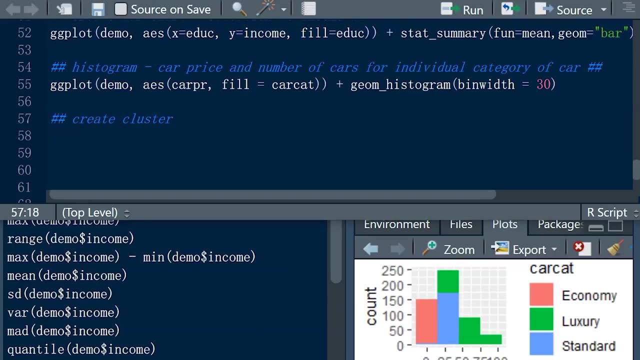 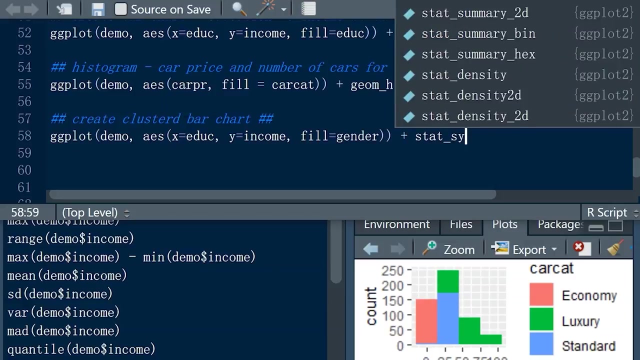 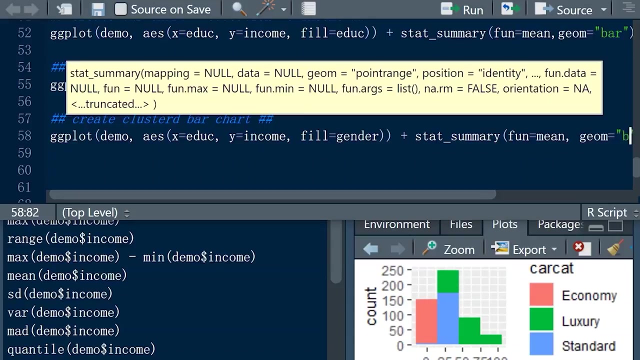 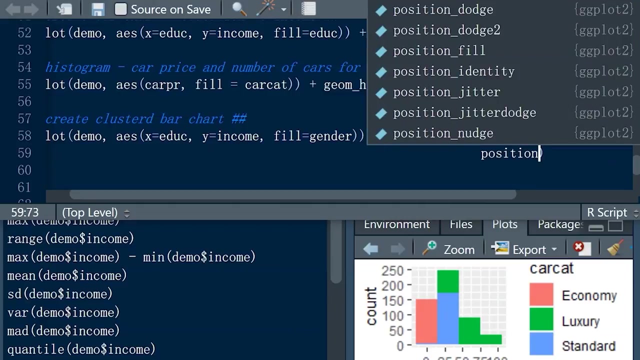 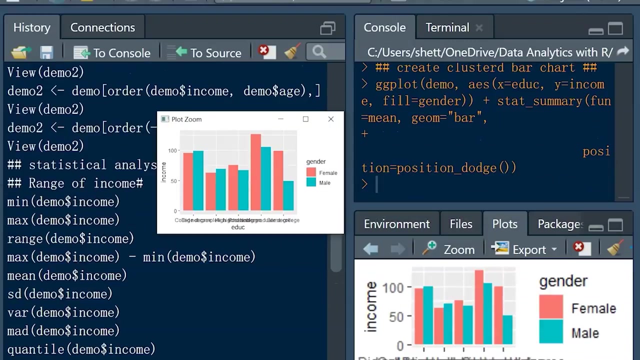 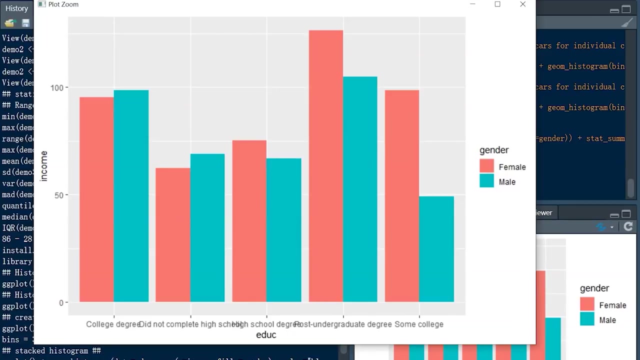 luxury and standard. this could be the starting car price of the luxury, luxury car category price of the luxury brands. now let us create a clustered bar chart. let's look at this visualization. in this visualization, as you observe, though, we have enabled fill equal to gender. in the aesthetic mapping, we do not. 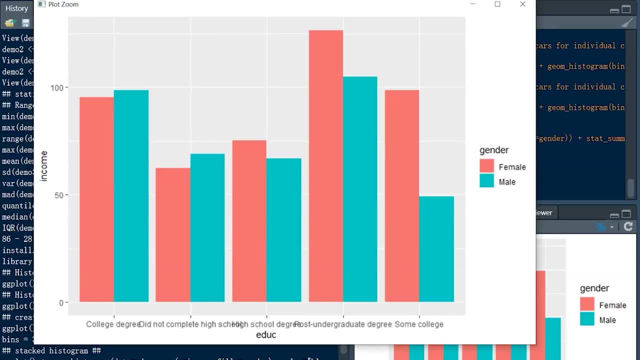 have the view in stack form, but we have the bars one besides the other. it is also because we have enabled a position called as position equal to dodge in the code. now what is the inside that we can draw from this visualization? as you see, post graduate degree with female gender is drawing higher average income as 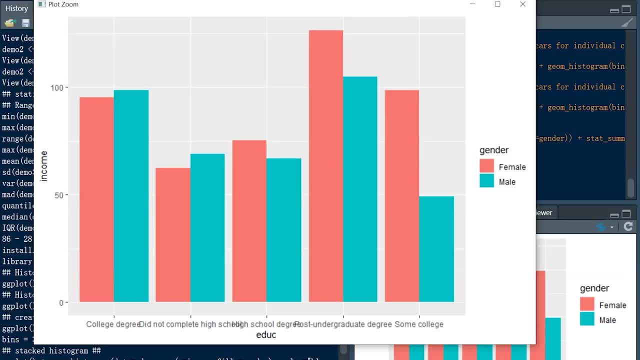 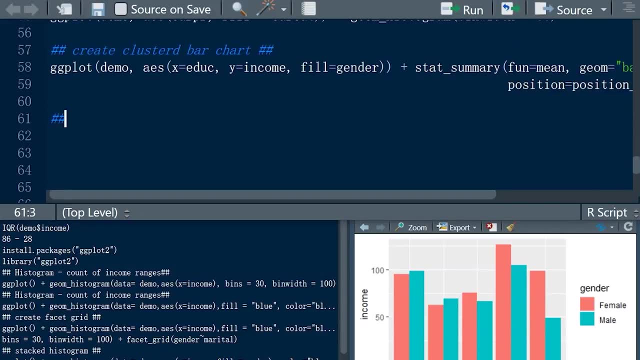 compared to any other education level. now let us see how to create a box plot for variable income across the genders. so the box plot can be enabled if there is a bivariate analysis to be performed on a continuous variable and a categorical variable, or multiple categorical variables with a continuous variable. 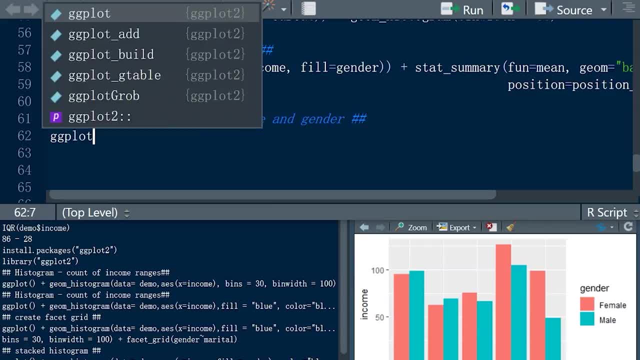 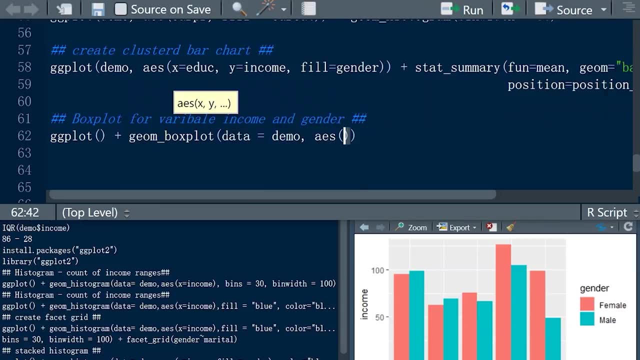 yes, the whole project is a system based on a single variable, so we can set the value of that variable on the random variable set and when we do that we can control how many variables we want to use or we may want to store them up as variables. we can also use a set of variables in the array of values for 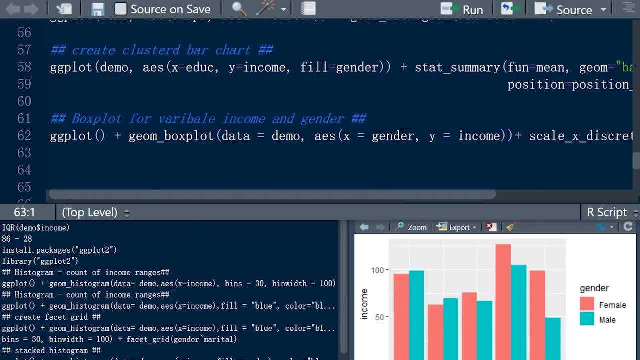 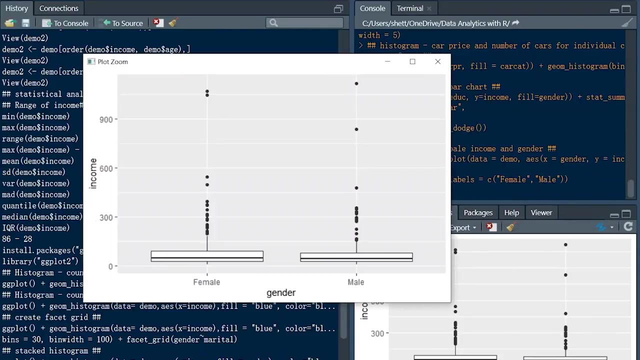 example, any number of variables for an array of values is important, because we want to make sure that all variables are equal. yes, and in any case, we want to also make sure that we are specifying any variables for any set of variables in the. Now let's look at this visualization. 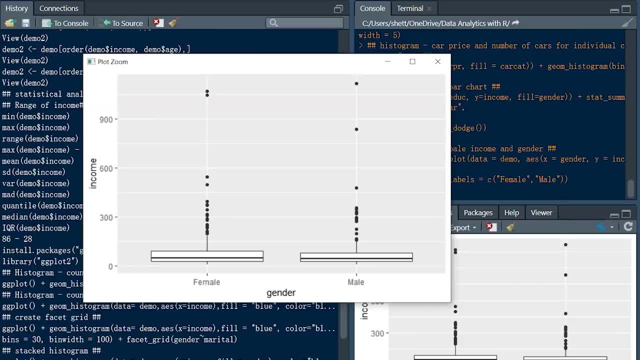 What does this say? We have data distribution of income for individual genders, that is, for female and the male, and we also notice outliers here. Anything above this whisker is considered to be outliers. It might make more sense if we also include some coloring for these outliers. 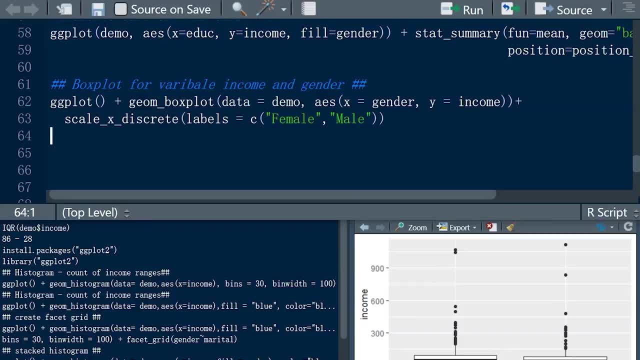 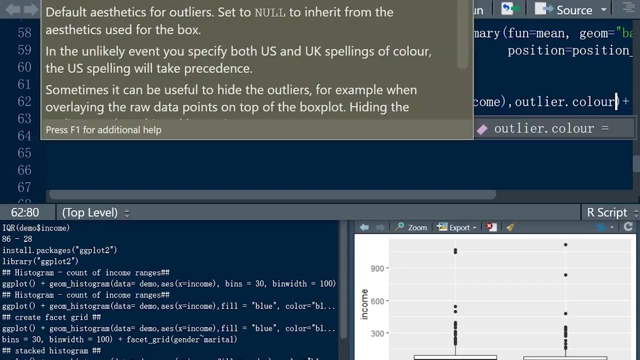 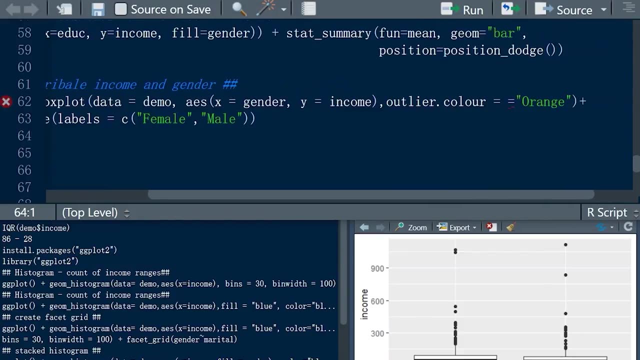 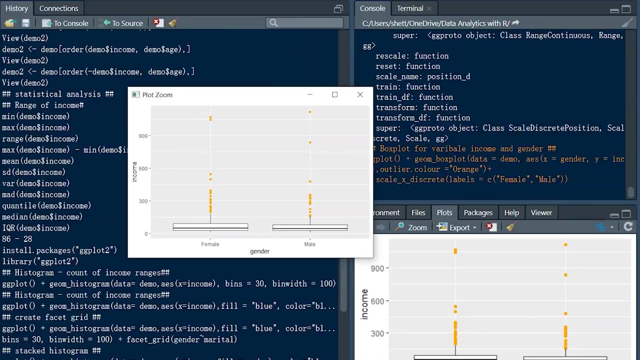 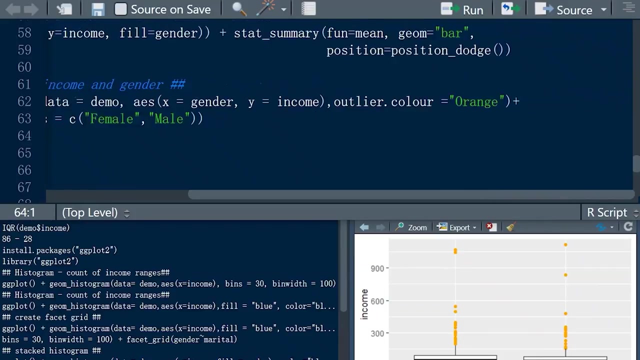 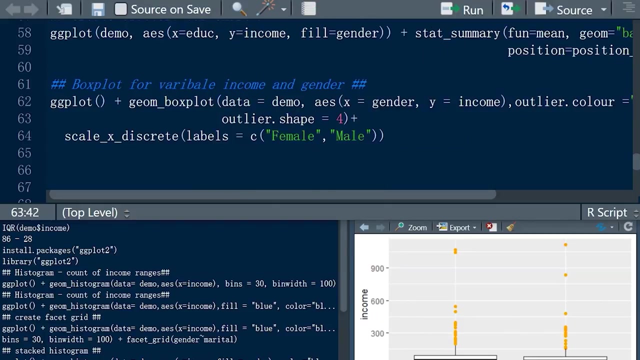 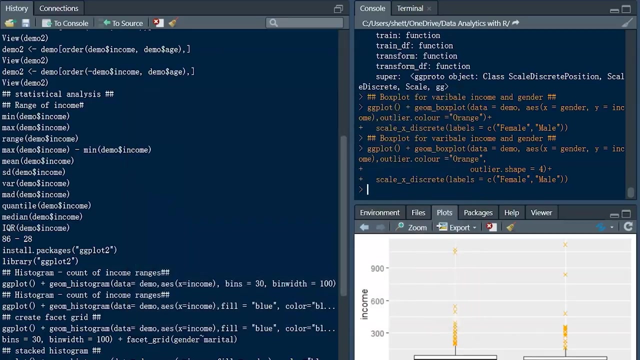 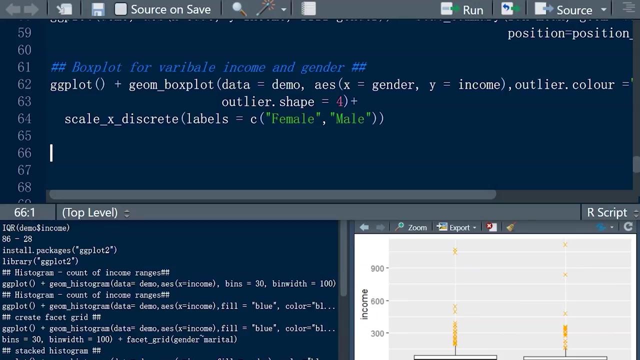 Maybe also enable shape. Now we have colored the outliers, Okay, And it's colored orange. Let's see if we can also enable the shapes. Now we have here the outlier color as well, the shape enabled. Now let us see how to enable a violin plot. 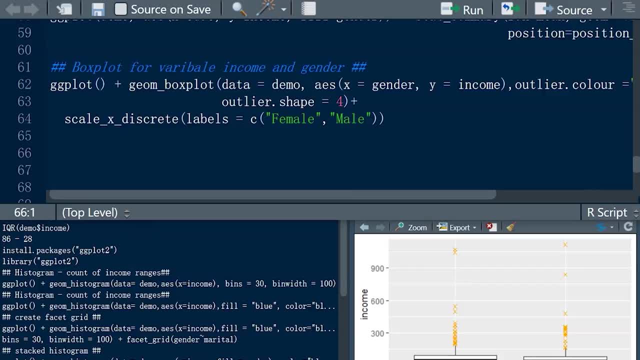 What is the utility of violin plot With a box plot? we understand the analysis and the distribution of the data points is to identify the outliers, to know what is the minimum value, what is the max, what is the median and what are the outliers. 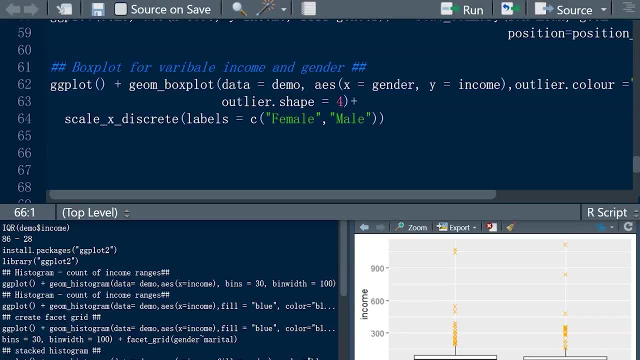 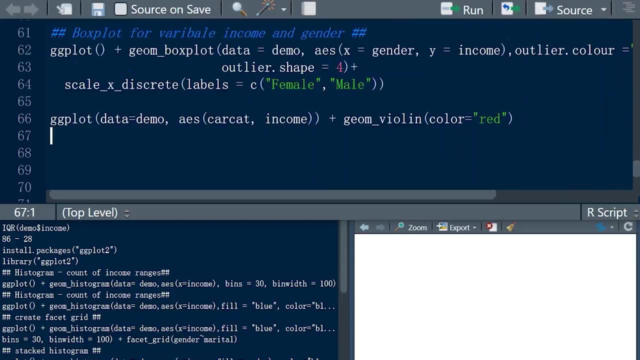 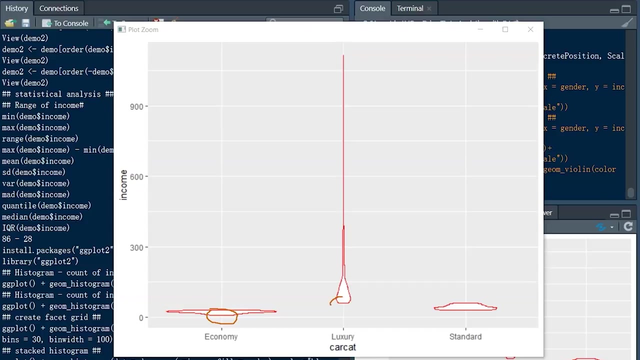 But what is the purpose of a violin plot? Let us have a quick check. Okay, As you observe, there is some concentration of data points in the bottom of every car category. However, the concentration is higher for standard car category as compared to economy and the. 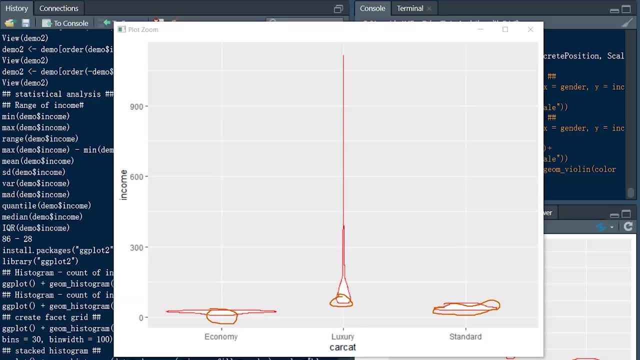 luxury. Now this is an interesting insight that you wouldn't have come across in box plot. The box plot is a very good representation for identifying outliers. However, violin plot will help you focus on the nuances which is not captured by the box plot. 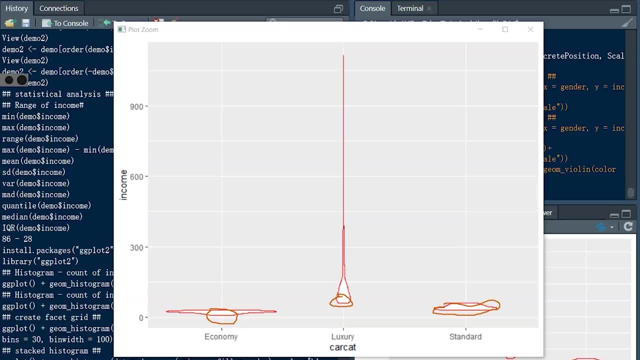 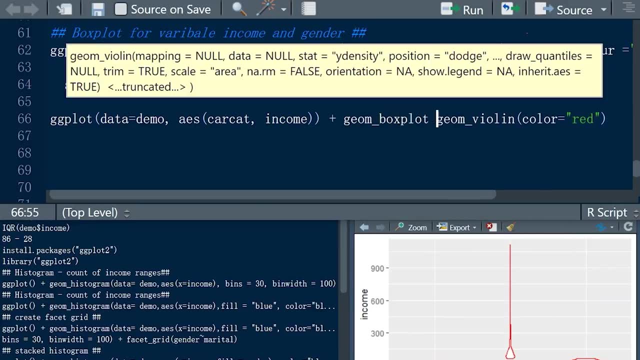 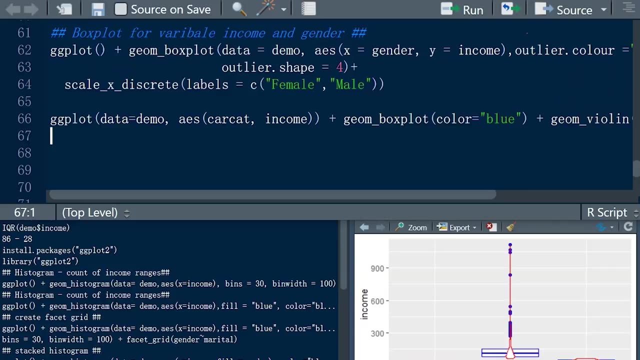 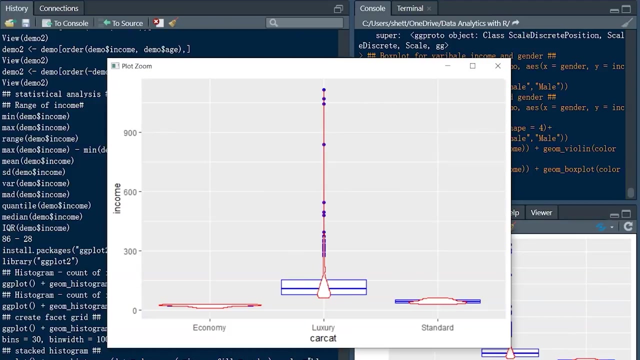 We can also simply combine the box plot and the violin plot together. Simply include this jaw object. Okay, Let's zoom this. Now you have a representation of box plot and the violin plot, both combined in a single visualization. Interestingly, you notice the outliers as well, the concentration in the bottom of this. 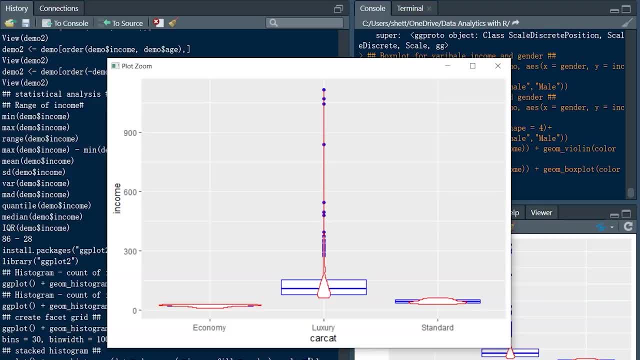 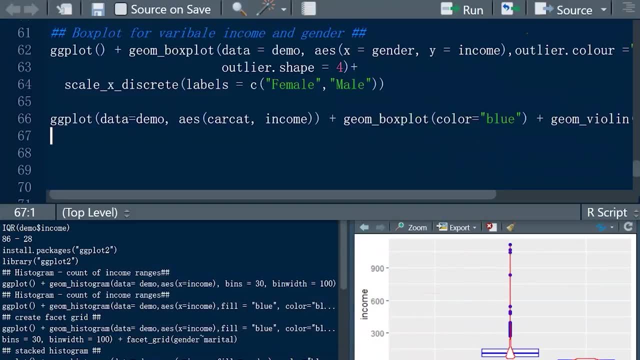 violin plot. So this could be some interesting insights that you draw and focus on these data points and understand what exactly is happening there. Okay, Now let's focus on the density plot, that is, density estimate of the histograms, rather than just viewing the frequencies. 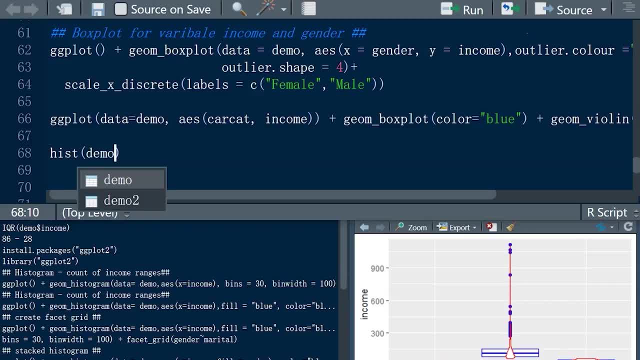 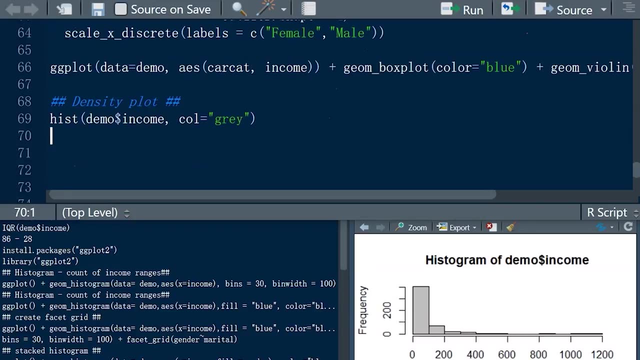 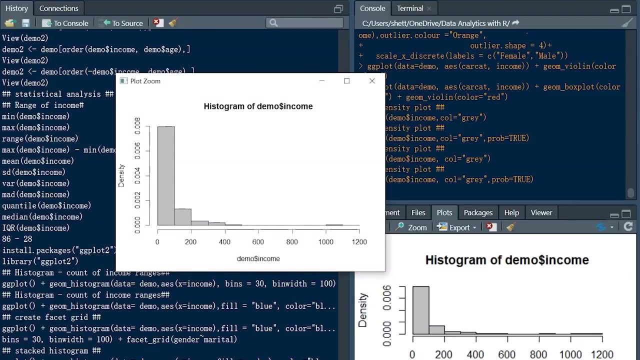 Now we see the frequency in the y-axis across the income distributions. How about enabling the probability as true, so that we enable the density instead of the frequency? So now we have the density in the y-axis, and in the x-axis we still have the income. 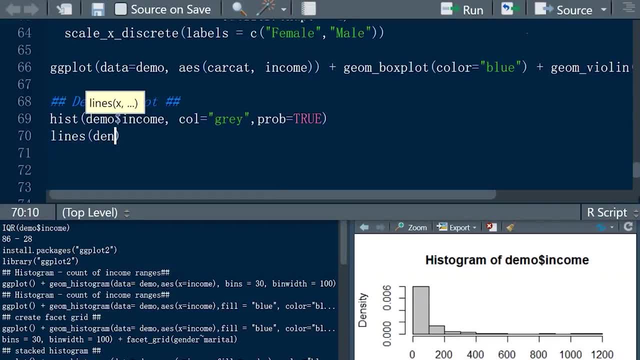 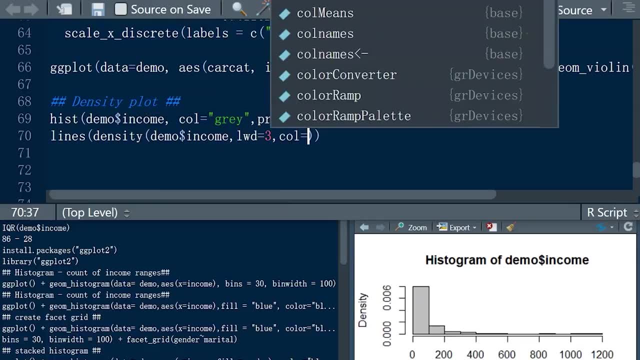 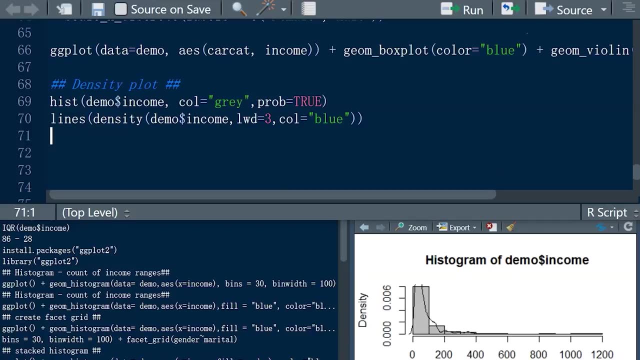 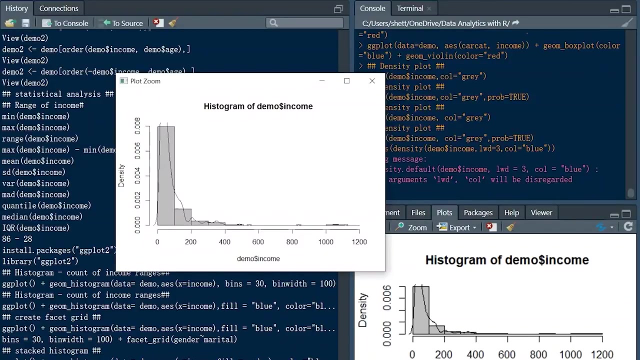 distribution. This is the way of also adding a line plot, which is a density plot. Okay, Now let's look at the histogram Now, as you observe, here, the density plot is not in the same level as the bar, So let us adjust this line. 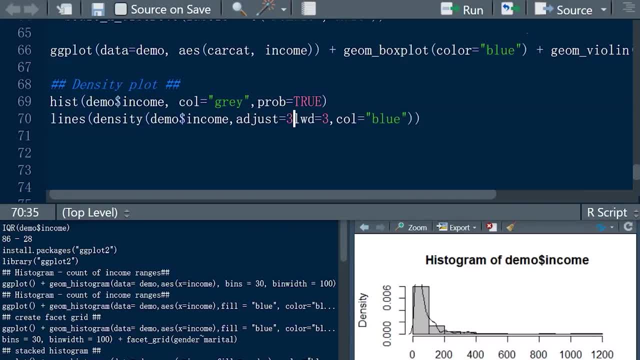 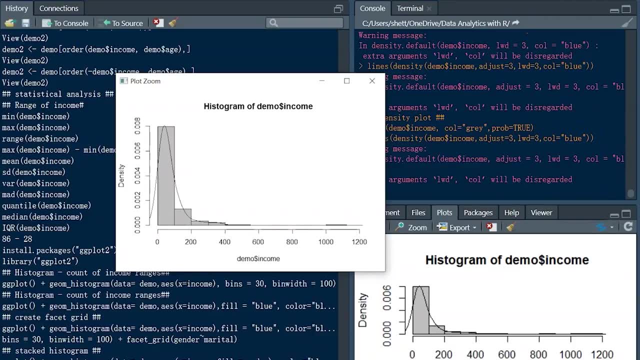 For this we will include: adjust, let's say, equal to 3. and now let us see how the visualization appears. Now the density plot is on the same level as the bar. Okay, Now let us see how to create a cross line. 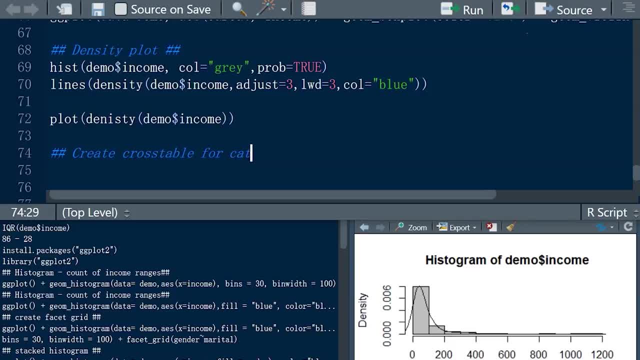 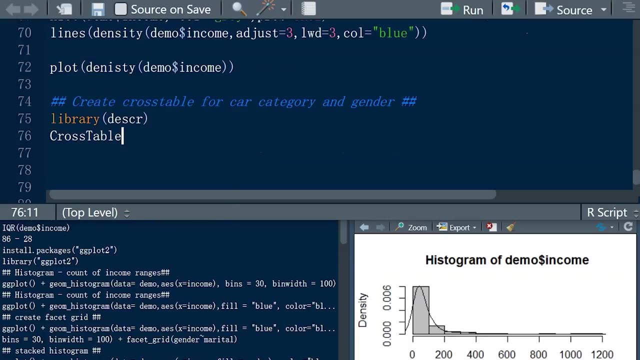 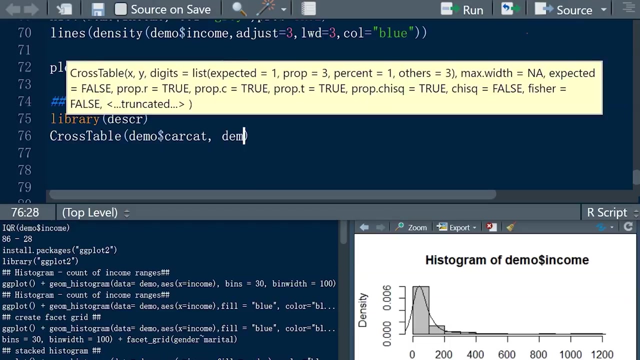 Okay, So let us create a cross table for car category and gender. For this let us call the library DESCR. Now let us create the visualization enabling cross table for car category and gender. Okay, Let's look at the visualization. 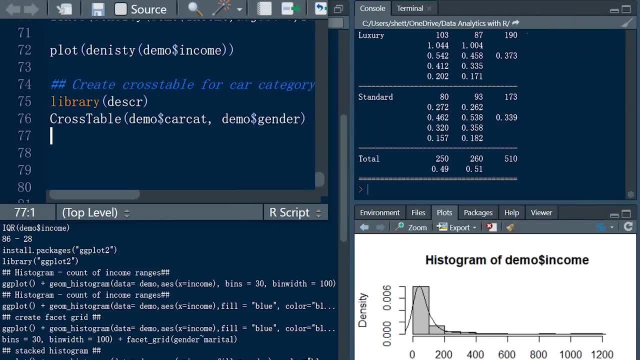 Okay, Now let us create the visualization. Okay, Okay, Let us look at the visualization and see how the visualization will result in console. Let us look at the visualization. Okay, Now let us look at the visualization and see how the visualization will result in console. 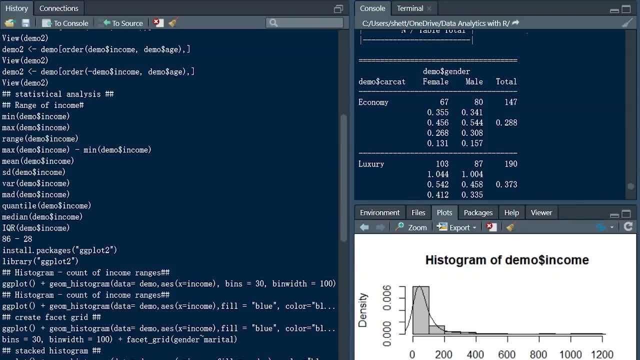 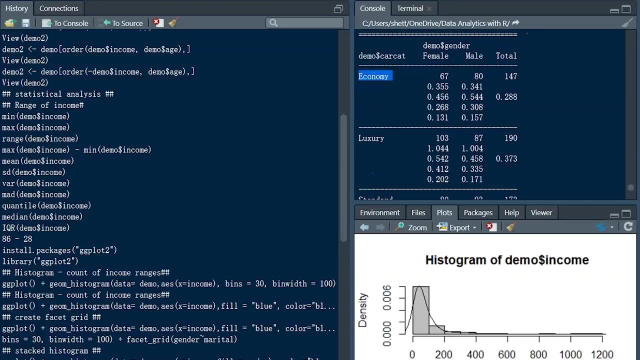 As you see here now we see the counts of the gender for individual car category. The values over here represents that there are 67 females falling within the car category economy and 80 males within the car category economy. And for luxury we see that the count of female is higher than the male as well. the proportions: 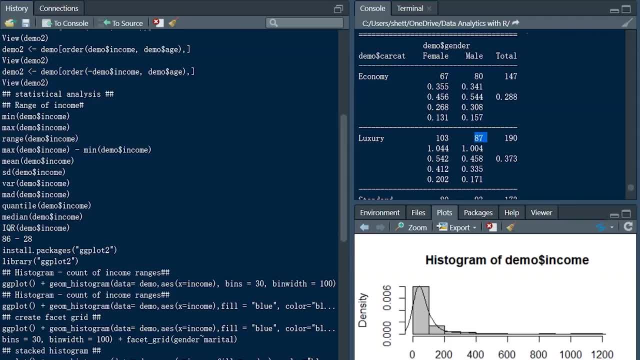 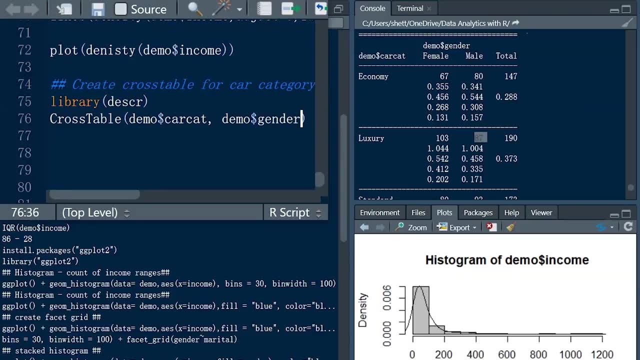 Now, how do you understand the main difference between the married and the divorced? In comes the advantage of the representation of the gender. What is the advantage of the representation of the gender? the proportions, Now. how do you understand what proportions are presented here? We may. 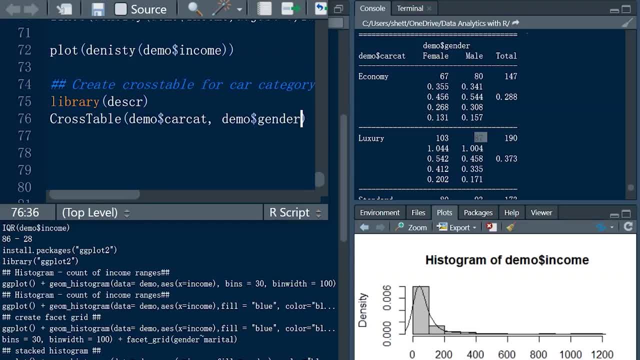 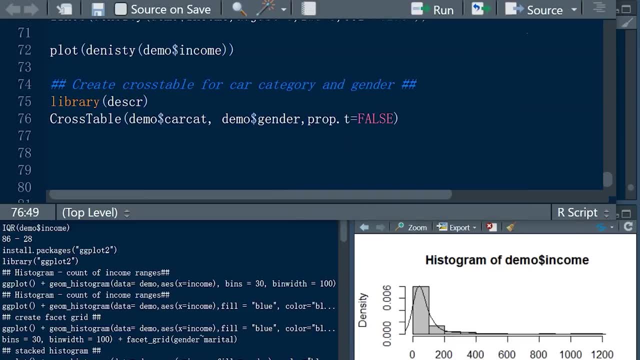 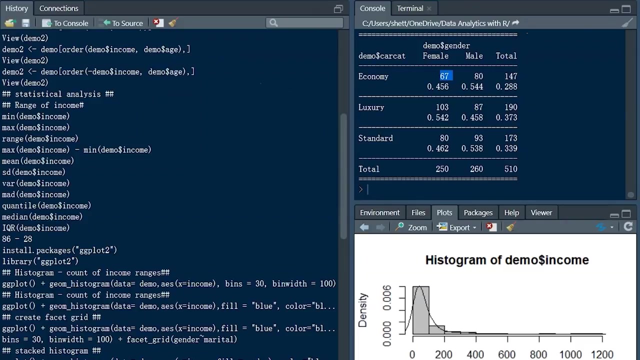 simply turn off some of the proportions, like the t-test, the chi-square, etc. Let us see how to enable that. Now let's look at the result. This looks better Now that we have the counts- the female counts and the male counts- across individual car category. we 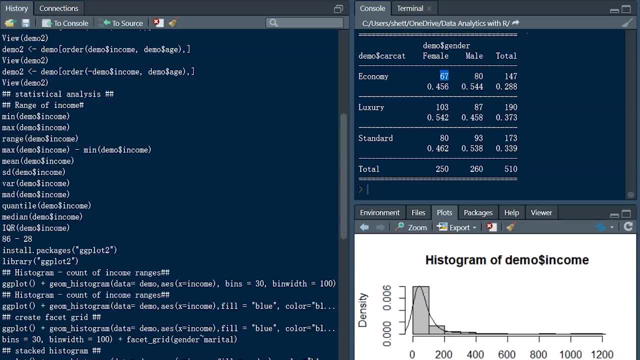 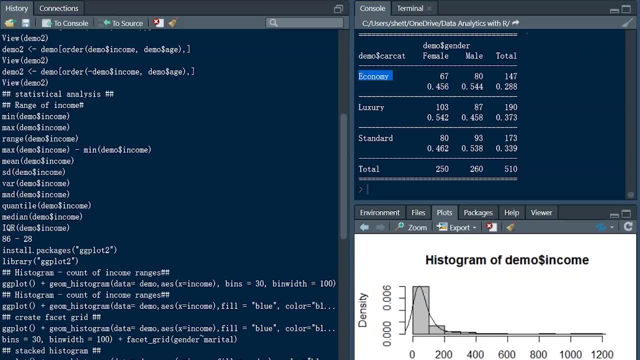 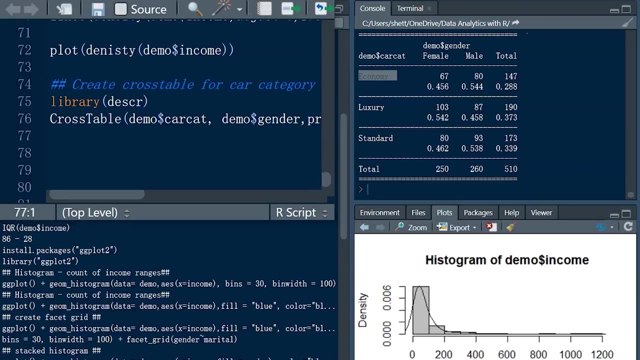 6% of female within the car category economy and 54.4 percentage of male within the car category economy, similarly across rest of the car categories. this kind of cross table, or a contingency table, is also helpful when you want to analyze the different categorical variables and 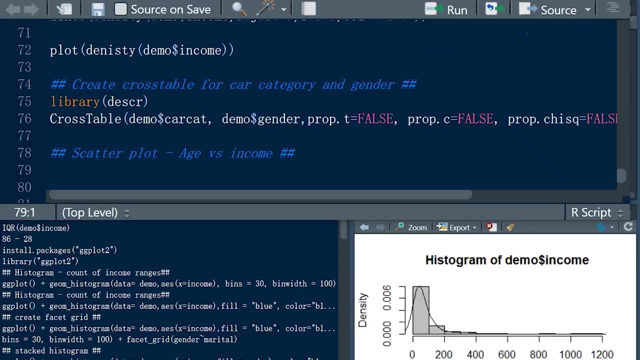 Identify the counts or the proportions. now Let us see how to use a scatterplot of age versus income. Scatterplot is a visualization used for bivariate analysis When you want to perform some analysis between two continuous variable at a data point level Rather than performing the analysis at an aggregated level, such as some or mean. 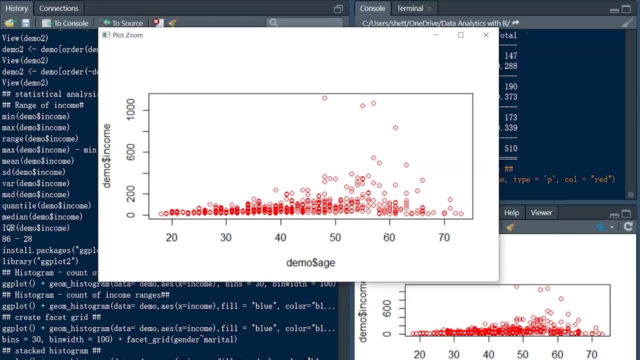 And now we have a scatterplot of age versus the income- age in the X axis and income in the Y axis, Though we do not see any kind of a positive correlation or negative correlation, But we still see some interesting insights over here. Some of the data points are pretty much scattered and much away from densely populated data points. 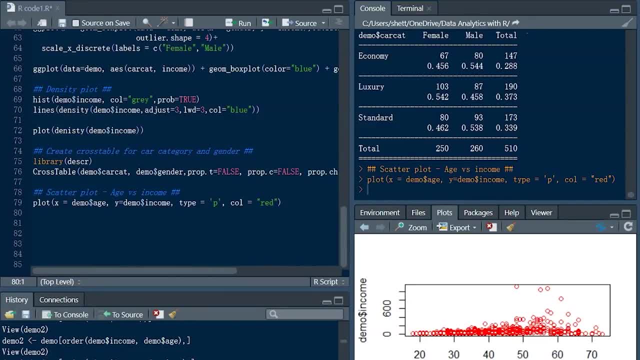 I hope the learning has been informative and interesting. so far we have covered the concepts of data analytics as well. we have performed some hands-on, doing some statistical analysis and also creating interesting visualization to learn more and further on data analysis with our. please watch the video above. thanks for.